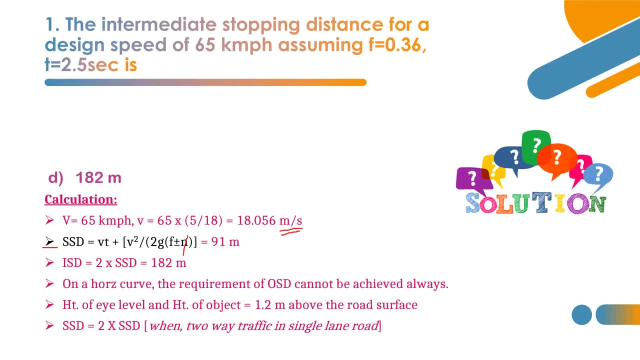 not mention anything about gradient. So this one is left out. this one is cancelled out. So v square by 2, g, f, 1.. So f is 0.36,, g is 9.81, v is 18.056.. So, substituting all those things, 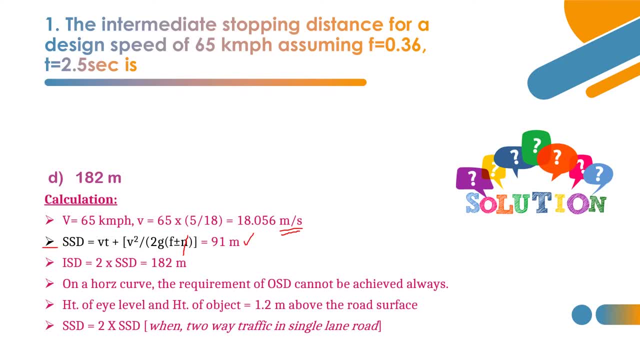 in this formula we will get. the answer is 91 meter. for SSD value. We are supposed to calculate only intermediates, stopping side distance. So ISD is given by 2 times SSD. So 2 into 91 gives 182 as answer. So option D is correct. Now let us see something more about ISD and SSD. 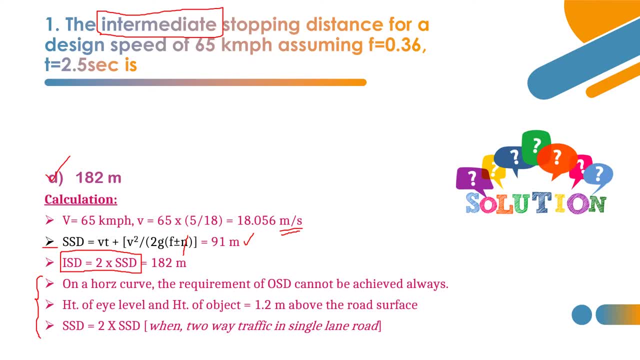 So on a horizontal curve. so why ISD is provided On a horizontal curve? the requirement of OSD cannot be always satisfied, So that is why we are providing ISD that is nothing but twice the standard. So we are providing ISD that is nothing but twice the standard. So 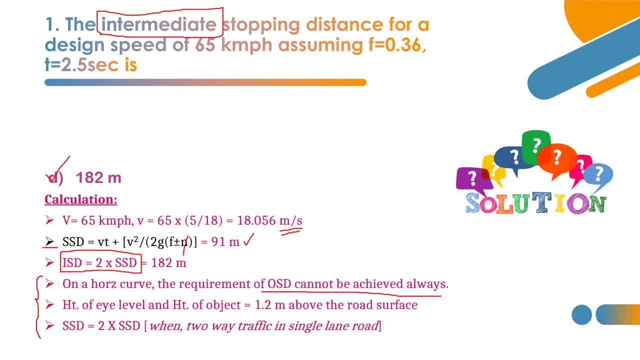 that is why we are providing ISD. that is nothing but twice the standard. So, on a horizontal curve, stop stopping side distance, SSD. And when it comes to ISD- height of eye level and height of object- both are considered as 1.2 meter above the ground surface or the above the road surface. 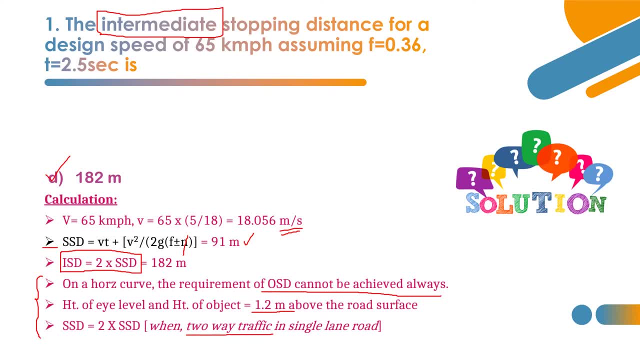 And when it comes to two-way traffic in a single lane road, SSD shall be twice that of the required obtained SSD value. So these are some important points regarding SSD and ISD. So ISD is nothing but twice that of SSD. SSD is given by this formula: VT plus V square by 2GF. 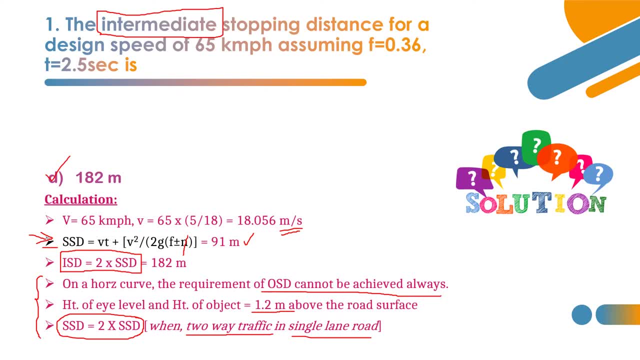 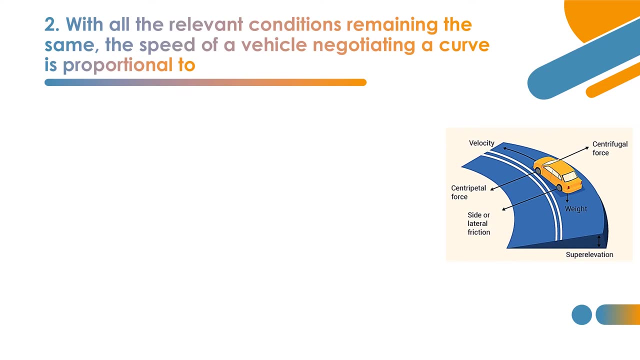 When a gradient value is mentioned, we have to substitute like this: F plus or minus N, N in percentage. Now let us move on to second question. Second question is based on a super elevation or we can say some centrifugal action in a. 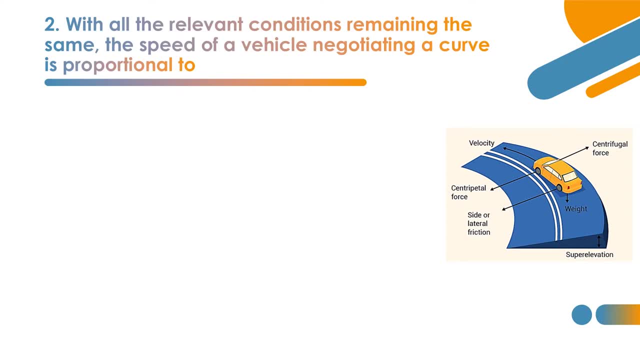 curve, with all the relevant conditions remaining the same. The speed of a vehicle negotiating a curve is proportional to: option A: weight of vehicle. option B: 1 by root of weight of vehicle. option C: root of the weight of vehicle. option D: reciprocal of weight of. 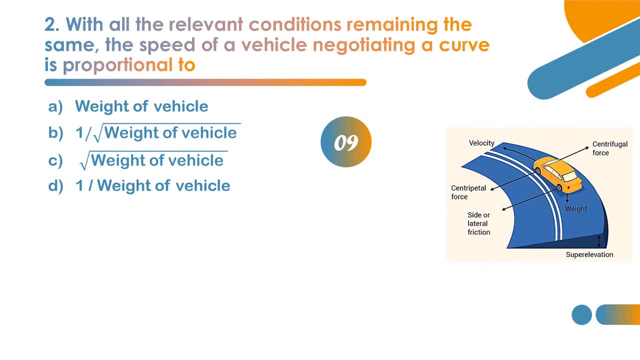 vehicle. So what is the correct option with respect to the speed of vehicle, with all the conditions remaining the same? What are the other conditions? Centrifugal force and radius of curve? What else? Velocity? So these conditions remaining same? What is the speed and weight relationship? So nothing but option B, reciprocal of root. 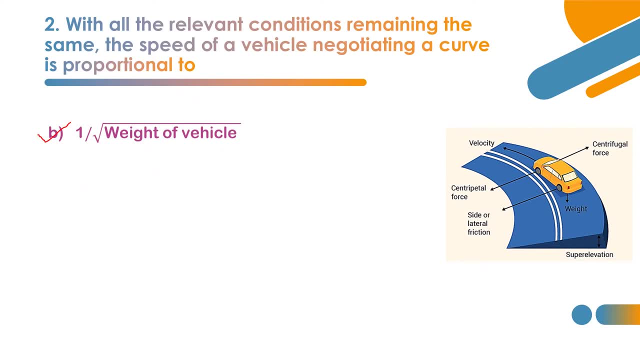 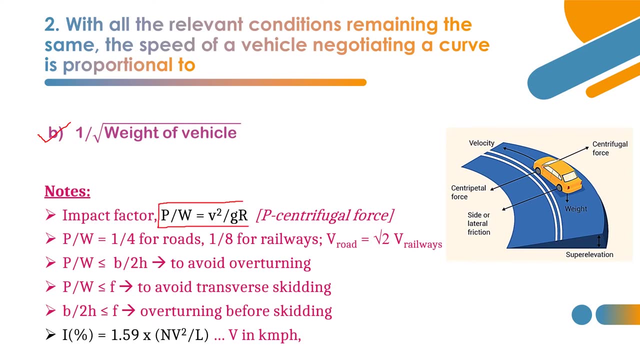 of weight of vehicle. Now let us see how it is obtained. This is how we are calculating. we are obtaining the relation between weight and velocity relation. So P by W is equal to V square by gr. This is nothing but impact. 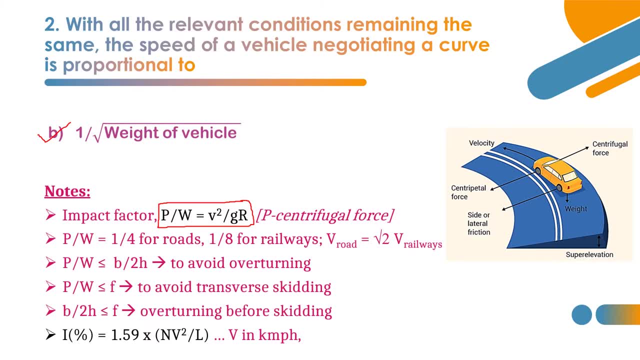 factor, or we can say centrifugal ratio, in by other name, and P is nothing but centrifugal force. So you can see in this diagram, this is the centrifugal force and opposing force is the centripetal force. So centrifugal force divided by weight of vehicle is equal. 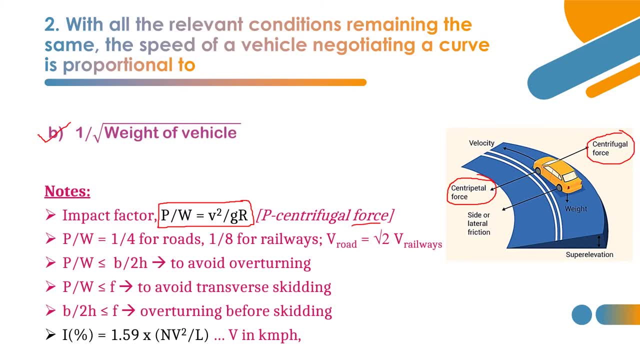 equals to equals to V square by gr. So this P by D, P by W is equal to V square by gr, And P by W ratio is nothing, but we can call that as impact factor or centrifugal ratio. So typical values for roads and railways is given as like this: 1 by 4 for roads and. 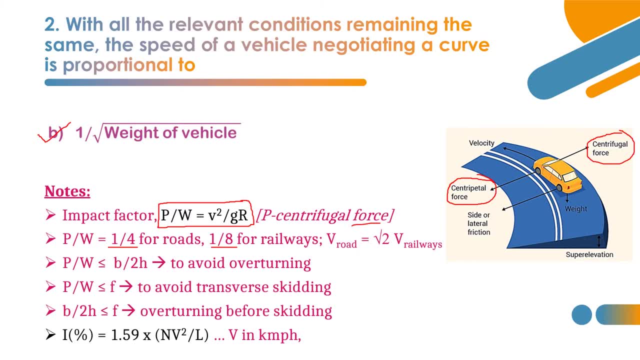 1 by 8 for railways. So if you substitute 1 by 4 here and calculate the velocity values by considering some radius of curve and G as 9.81,, you will get one value and that value related to railways. we get the answer as V square by gr. 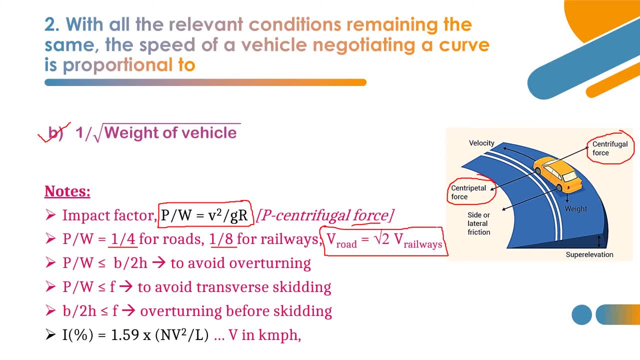 that is, maximum speed, of speed in case of road, will be equal to root, 2 times the root, 2 times that of railways. So this is some an observation. this is an observation when we substitute the value of p by w, value that is impact factor. and let us say something more about it. when p by w, 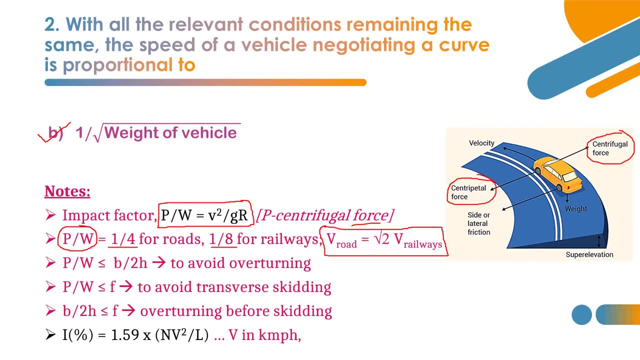 is less than b by 2 h, then it to avoid actually overturning we the relation should be like this: p by w shall be less than or equal to b by 2 h. So what is b? b is the width of vehicle, h is the. 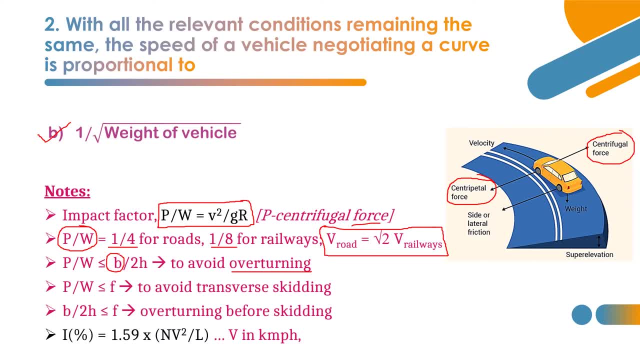 height above the ground. So p by w shall be less than or equal to b by 2 h, then only we can avoid overturning. and the p by w ratio shall be less than or equal to f, then only we can avoid overturning. So this is the relation. So this is the relation, So 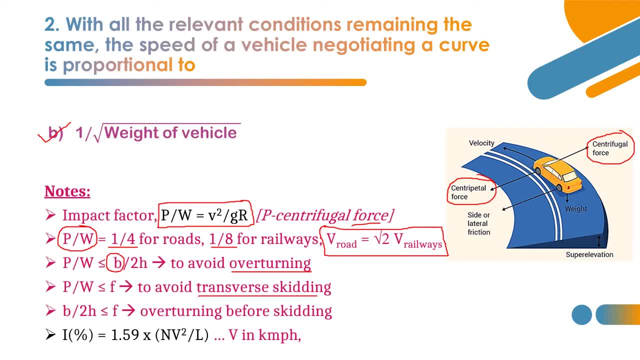 we can avoid transverse skidding or lateral skidding. if b by 2- h is less than f, less than or equal to f, then high amount of friction is there. what that? what does it mean? overturning will occur before skidding occurring. So overturning before skidding: b by 2 h less. 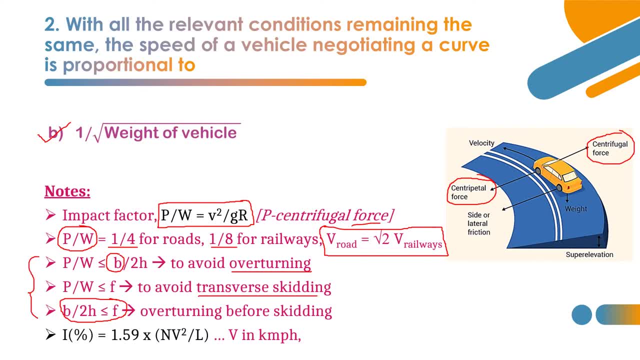 than or equal to f. So these are about some relations between impact factor and the and the corresponding b by 2 h value. to avoid overturning Skidding and like this, and another important formula is formula for impact factor, is this one: 1.59 into n v square by l. So n is nothing but deviation angle, that is algebraic difference. 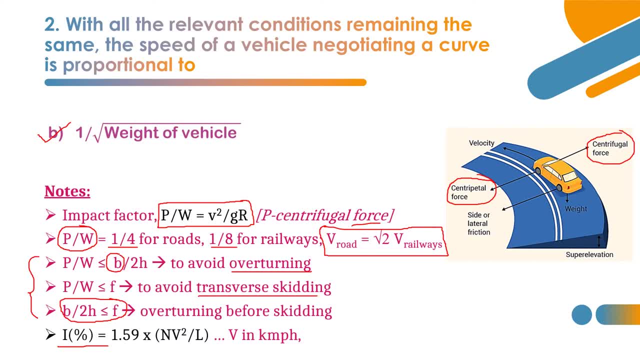 between the gradients and v. here v is written in capital letters. whenever v is written in capital letter, then we, then the unit will be unit would be kilometer per hour. when v is in small letter, then that unit will be meter per second. So this is how we have to follow the sign. 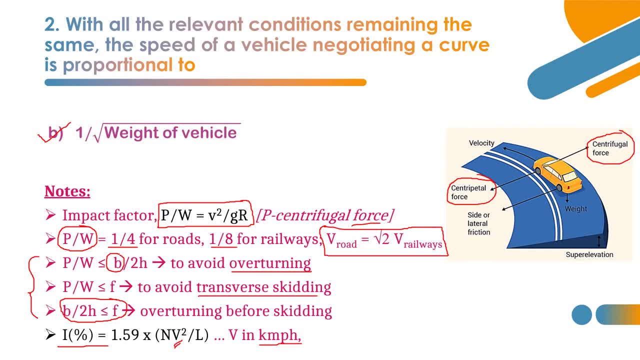 conventions. So here, 1.59 into n v square by l is the impact factor in percentage. this is one important formula that are used, that is used in various problems. So these are all about the impact factor. p by w is equal to v square by z r. Now let us move on to 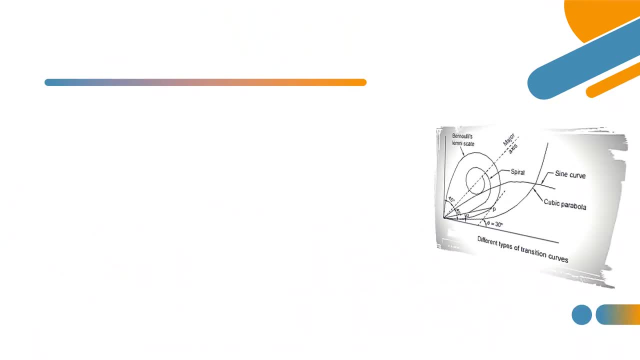 third question. Third question is based on transition curve. the standard equation of cubic spiral transition curve. There are many types of curve here. you can refer in this diagram: spiral cubic parabola, Bernoulli's lemniscate like this sign curve. there are many types of transition curves available. Now we have to find the 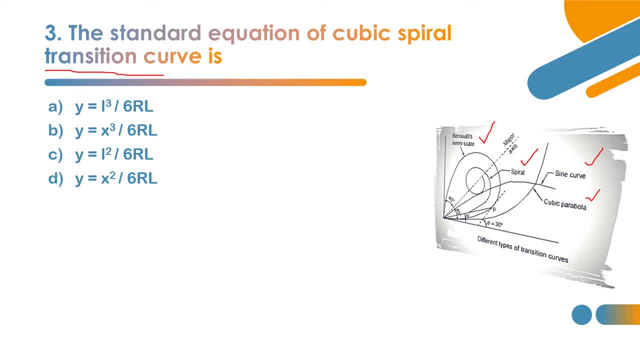 option for cubic spiral transition curve. standard equation for cubic spiral transition curve. So, among the four options, what is the correct equation For cubic spiral transition curve? So the correct equation, or cubic spiral transition curve, is option a. y is equal to l cube by 6 r l. Now let us see more about the other. 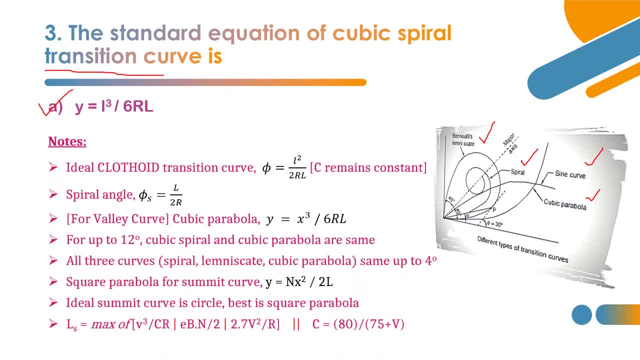 curves. Actually for transition curve, ideal curve is clothed or we can say spiral. that for that equation, for the spiral, the equation goes like this: pi is equal to l square by 2 pi rl. pi is nothing but the angle. this angle is this angle they are denoting. pi is equal to l square by 2 pi rl. why transition? why ideal? 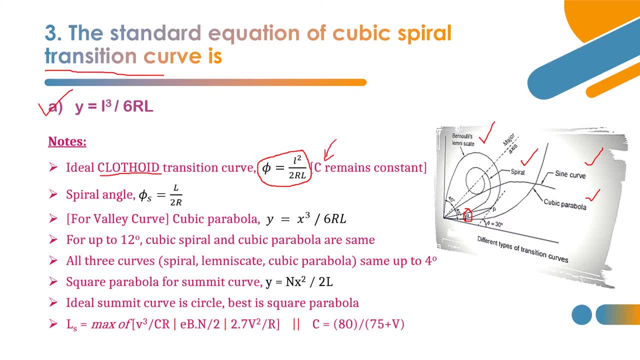 transition curve is clothed because c, this c remains constant. what is c acceleration? radial acceleration. so radial acceleration: c value meter per second square per second rate of change of radial acceleration. that remains constant in case of clothed transition curve. so that's why this clothed or spiral curve is identified as ideal transition curve and the spiral angle is given. 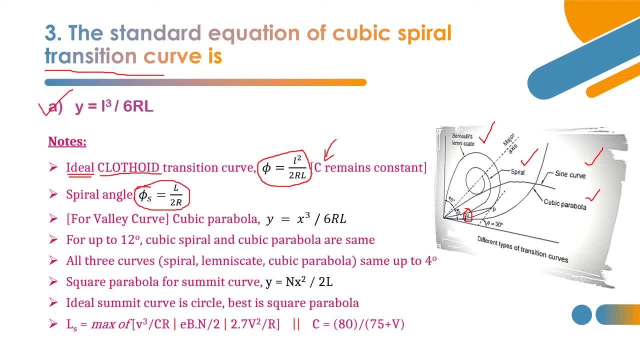 by this formula, l by 2 r, and for valley curve. and let's see some other curves. with respect to the function for valley curve we use q and that equation is given by: y is equal to x, cube by 6 rl. so y is equal to 6 cube, x cube by 6 rl. 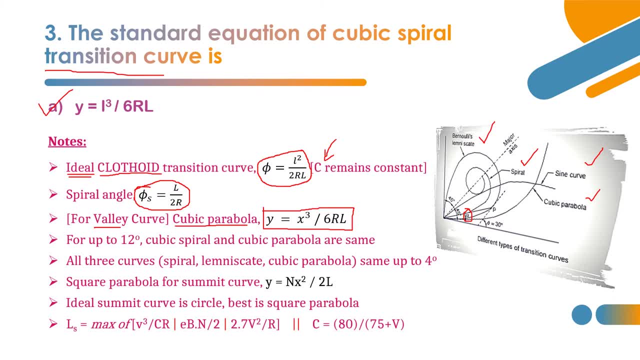 is the valley curve equation. cubic parabolic valley curve equation. so x cube 6 rl, here l cube 6 rl. so there is some difference. this is x, x axis value, this is the x, but here l l is nothing but length. so cubic spiral transition curve is l cube by 6 rl. 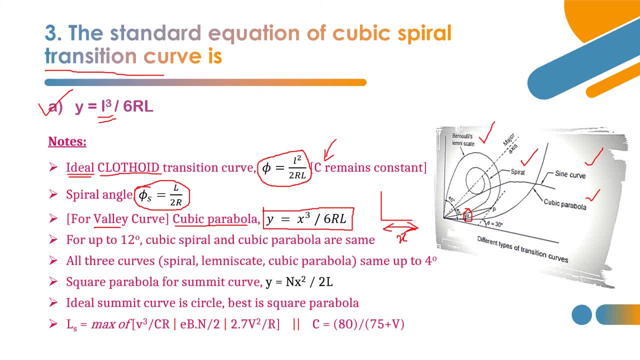 when it comes to cubic parabolic valley curve, it is x cube by 6 rl. now let's say some other point for up to 12 degree, cubic spiral and cubic parabola are one and same, so this formula and this formula are same up to 12 degree. 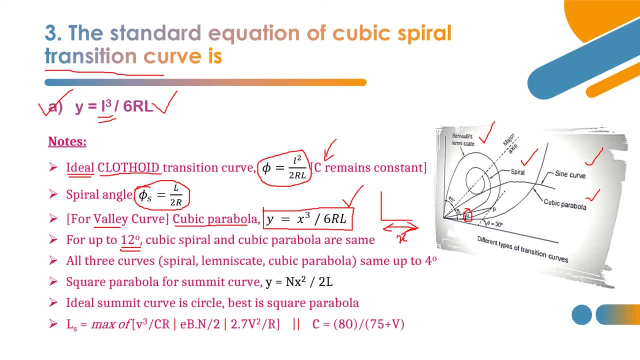 taco. so basically it's kind of like sum. the length of the kissing pattern is same as 1 and the co position of one nut, one nut extra 3 qu lleva is equal to 4 новые, as this is fah degrees. so up to 4 degree deviation, these three curves behaves one and same. 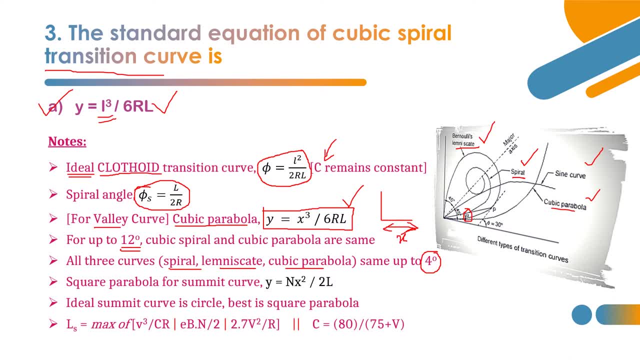 beyond that, only these three, has unique significance. and for summit curve, the curve adopted is square, parabola: square parabola is for summit curve, cubic parabola is for a valley curve. so this is the summit curve and this is the valley curve. ideal summit curve is circle, but best suited is square. 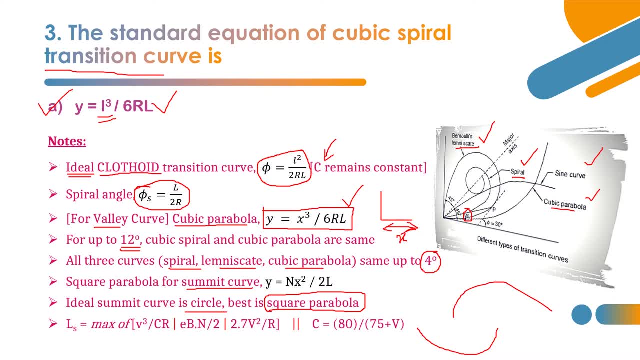 parabola. why ideal summit curve is circle? why ideal summit curve is circle? because side distance available throughout the curve is constant. so that's why circle is the ideal shape for summit curve. but but due to good riding qualities and simplicity of calculation, the best curve for summit curve is square. 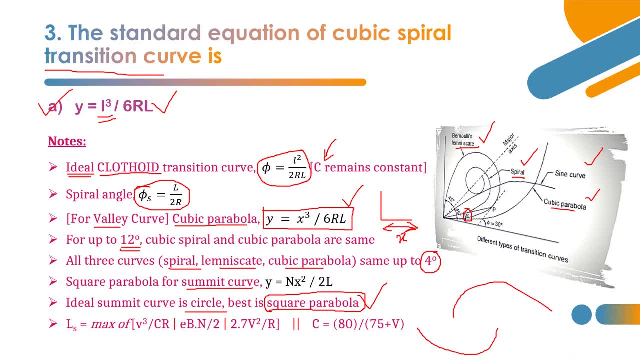 parabola. ideal is circle, best suited is square parabola. there is difference between best and ideal when it comes to ideal curve. it it is side. it is different. it depends on side distance criteria. so that's why circle is the ideal summit curve. but in case of comfort, best ride quality and the simplicity in 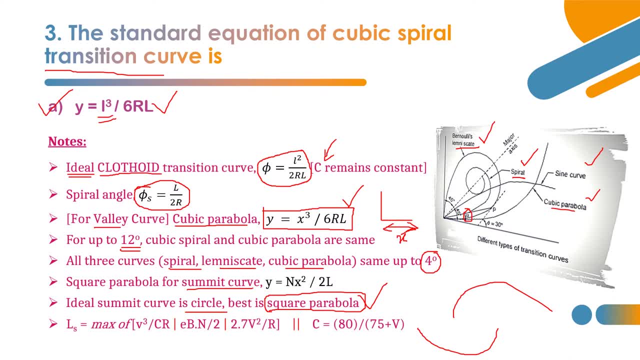 calculation: square parabola is the best one. so there is one difference. and what is the length of transition curve? how that will be calculated by using this formula: a less is nothing but maximum of V cube by C R. here V is in small adult. that means which the velocity value has to be substituted in meter per. 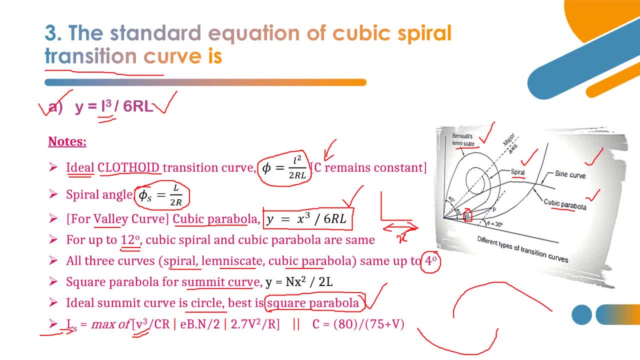 second nearby C, R. C is nothing but write of radial acceleration. that will be given by using this formula: 80 by 75 plus B. here V is in capital letters. that means kilometer per hat. another fairness: e be into n by 2 and aYenter be ugTimely the과�abd by yEntre. 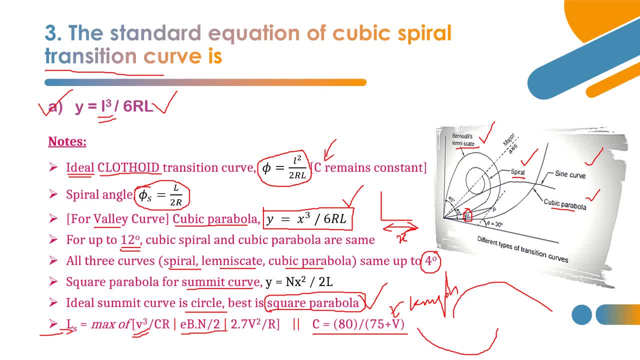 2. so what is e super elevation? b is nothing but width of highway, including the extended width or widening. so there is one concept of widening of curves, so that is included in this capital. b into n, n is nothing but rate of super elevation. this will be respect corresponding to the 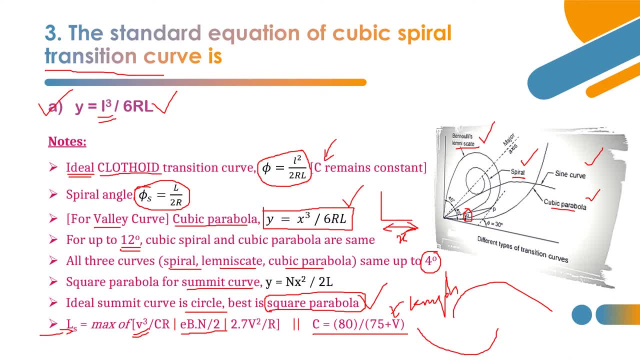 curves, that is, that curve is in high flat road or that curve is in built road or that goes in the highway or hill, hill roads. so that depends on. if it is in mountainous road, then n will n will be 60. if it is in plain, if the highway is constructed in planned areas, then n will be 1. 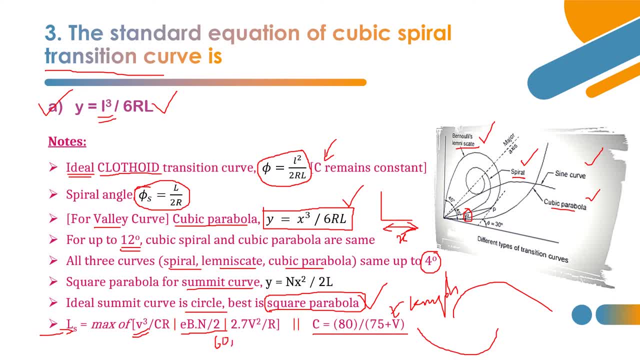 1 from 150. so for a mountain it is 60, for plane it is 150 and for built up areas it will be 100. so these are some typical n values. that is nothing but rate of introduction of super elevation. so it is n will be 60 for mountain. 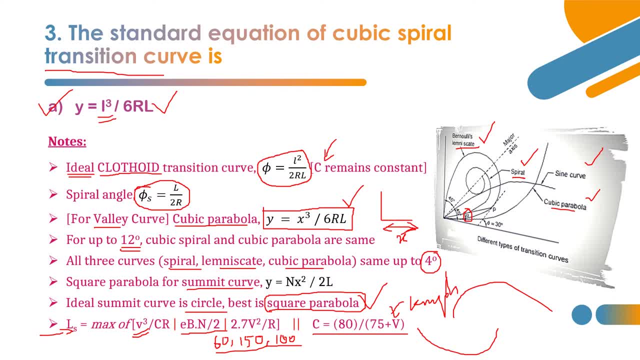 150 for plain areas, 100 for built up areas, and this by 2. e b n. divided by 2, that will be come when the curve is, then the pavement is rotated about center. when the pavement is rotated about inner area, then this by 2 will not come, only e b n. and another criteria is 2.7 v square by r. here v is in. 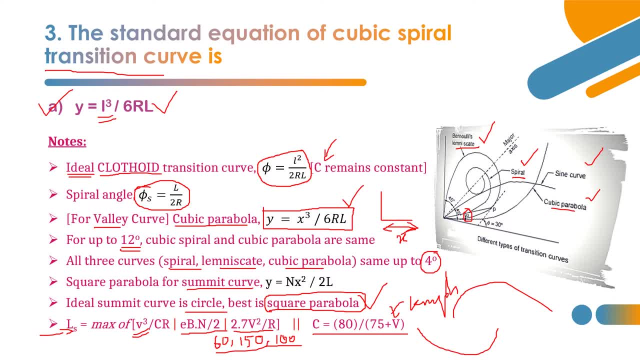 capital letter. that means velocity should be substituted in kilometer per hour and 2.7 v square by r is based on irc codal provisions and 2.7 v square by r is for plane and when it comes to hinded in the slope by x Model. Whatever and is measured is próxima. 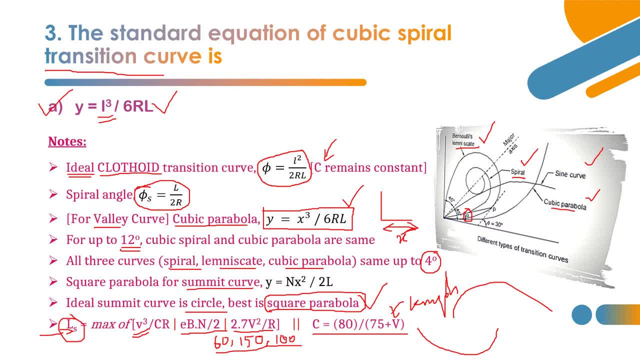 Then in today's graphic examples, we focus on a. we will be going into an important part of discussion about the change of height Once a deine time when w equation value is converted from la- We are going to believe to be slightly better- and c is capitalized by using the formula t by 75 plus v. now let us move on to 4th question. 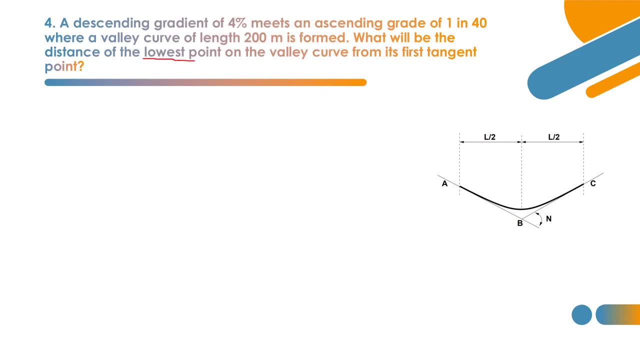 This is based on the valley curve. we have to find the lowest two points: the descending gradient, kirchoff, which must be maintained and is the Standard at the highest point. we then said that the train comes from lo and e, most of the places in the north of many states and the terrain. 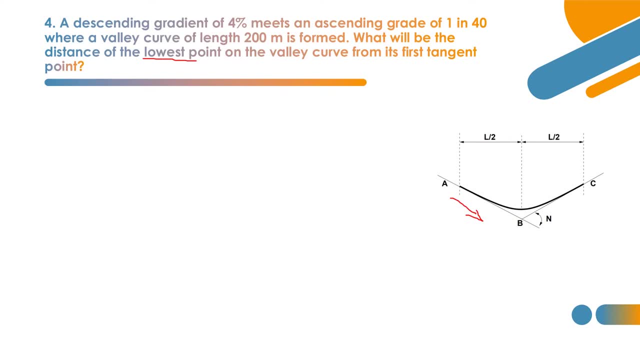 We were to find the points in both the direction of the warmth, in order to reached enormous low contact, and to the top sea and the trench, the bractte, we. we also know that nature of take away the height of 4 percentage meets an ascending gradient of 1 in 40, where a valley curve of length. 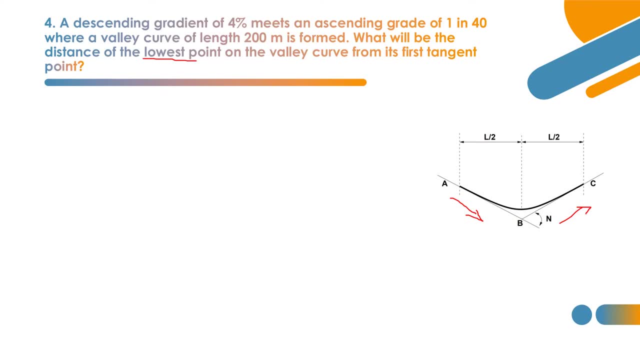 200 meter is formed. So length of valley curve, they have given What will be the distance of the lowest point on the valley curve from its first tangent point. So this is the first tangent point. So we have to calculate the distance between that lowest point and first. 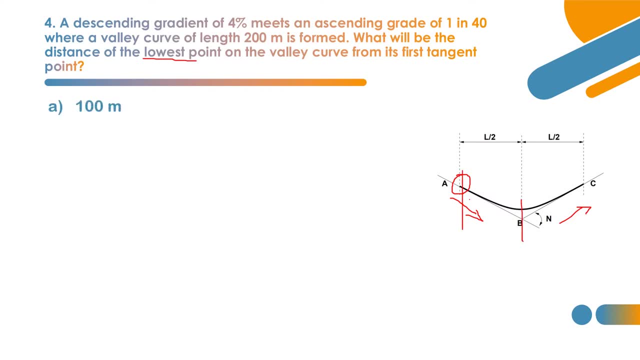 tangent point. So how to calculate that? Option A: 100 meter, option B 111 meter, option C: 125 meter, option D: 118 meter. So we have to calculate the distance of lowest point on the valley curve from its FTP first tangent point. This is one simple formula we have. 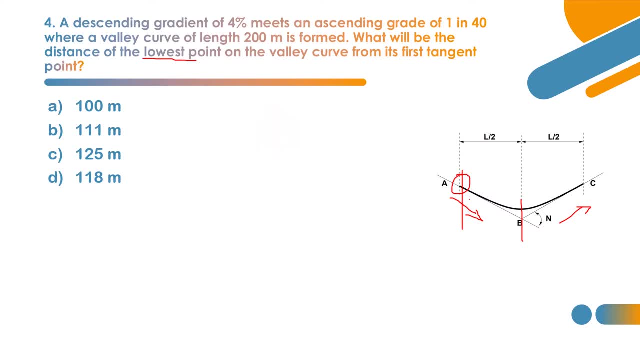 to remember so that we can find the answer for this question. So option is option B: 111 meter. Now let us see how it is calculated. X is equal to capital L. that is the length of the curve, 200 meter into n. 1. divided by 2 n, n, 1 is: 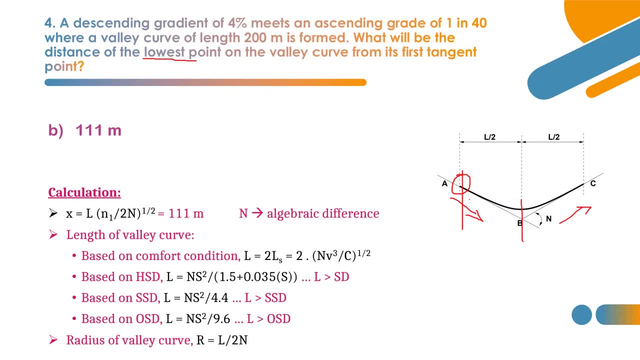 the descending curve descending gradient, sorry, not curve, descending gradient. So L is nothing but 200.. So we have to calculate the distance of the lowest point on the valley curve from its first tangent point. If we think of the above two expressions, as you can see that, the shadow is there. sorry, it is directly like that. So at this distance above it it is not a shadow. So let us see the distance at the point. it is slightly higher. We need that stayed in place, that at this place, at this location. So, for example, the governments. 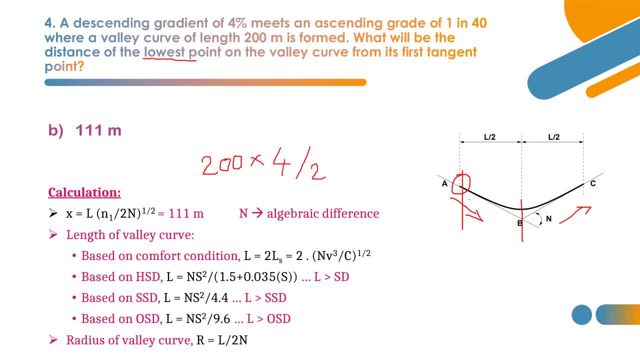 give this code looks like this. The governor asks about its equinox. What happens here? So we write theкоordinations of z equal to z 1 by z s into n 1, because this is the istantial sense. So we get the actually constant. Then why? 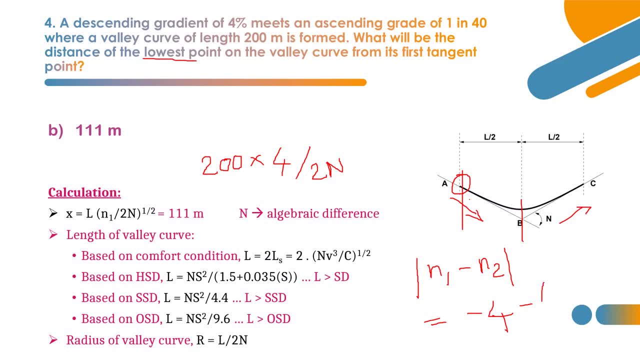 is this coefficient celebrate? n2 is an ascending gradient. So plus what? 1 in 40. So 1 by 40, that is it. So the answer is the capital n value. So substituting all those things in this formula, we get 11 meter as the. 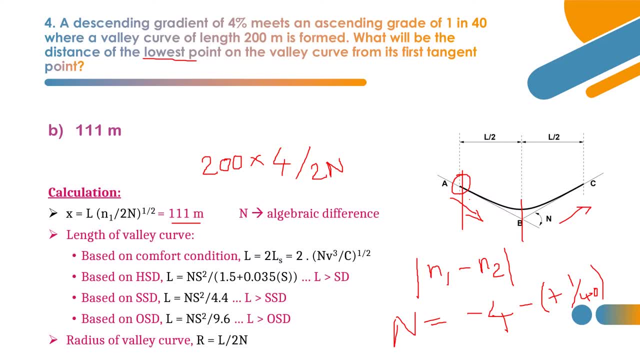 answer. that is nothing but distance of the lowest point on the valley curve from its first tangent point. x is given by. x is equal to l into n1 by 2, capital n power 1 by 2, or we can say root of n1. 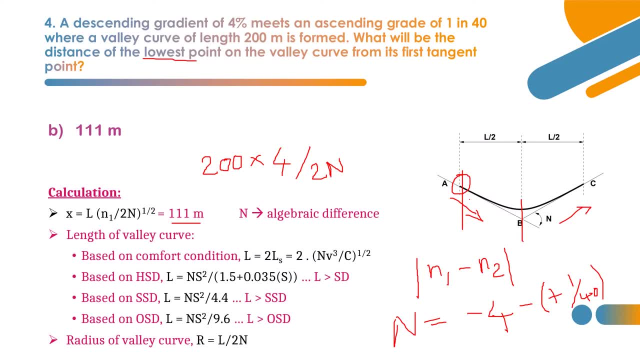 by 2n. Now let us see more about a valley curve. How length of valley curve is measured? based on comfort condition, headlight side distance, ssg and osg From based on comfort condition. this is the formula: l is equal to 2 times ls. ls is transition curve length. length of transition. 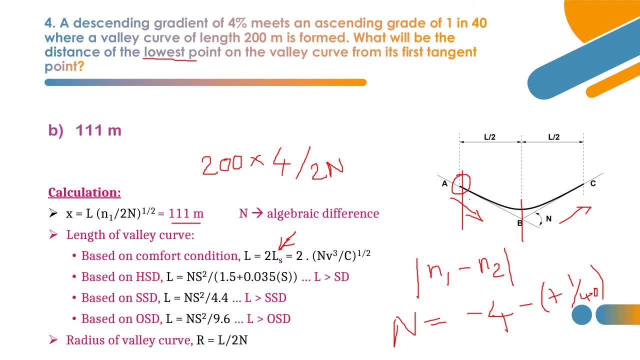 curve And 2 into nv cube by c. n is algebraic difference of angle or deviation, deviation grade. nv cube divided by c, c is the what meter cube per second cube. that is nothing but rate of radial acceleration. So nv cube by c, whole power 1 by 2 or root of nv cube by c. So this is how we have. 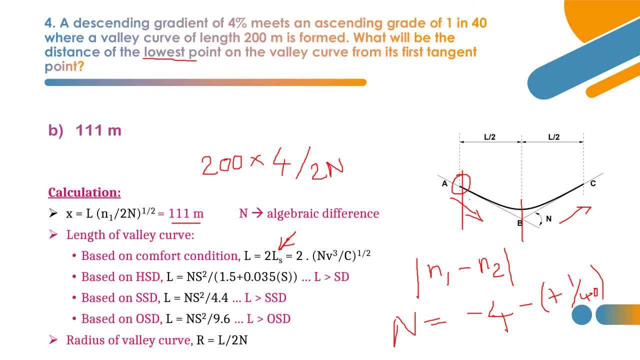 to calculate length of valley curve based on comfort condition And based on hsg l is equal to ns square. So we have to calculate length of valley curve based on hsg l is equal to 1.5 plus 0.035, 1.5. 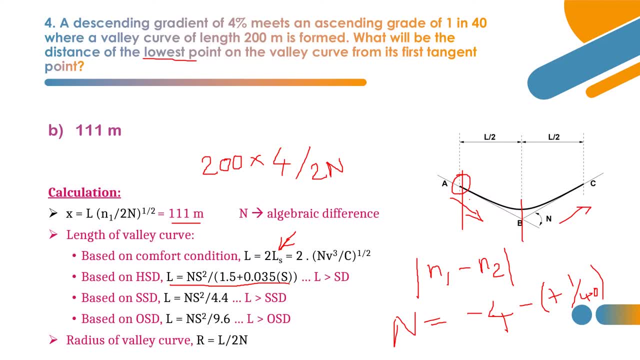 plus 0.035 s. s is nothing but side distance Only when length is length of valley curve is greater than side distance. If length of valley curve is less than side distance, then formula will get changed like this: to: s minus the reciprocal of this. How to how to calculate that l is equal to. 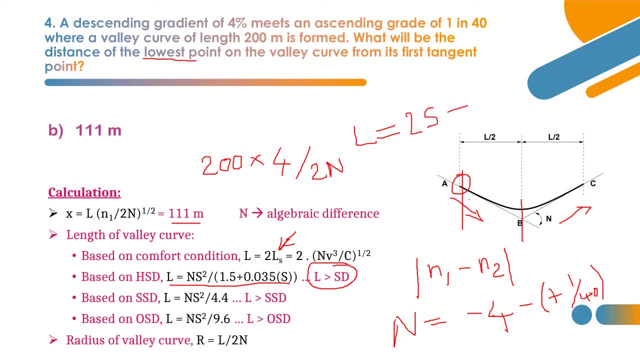 2s minus reciprocal, So 1.5 plus that 1 0.035 0.035 value divided by n. So this is how we have to calculate when l is less than sd. So when l is greater than sd, we have to adopt this. 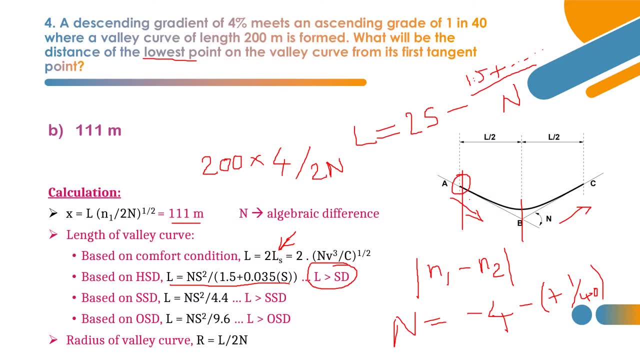 formula: l is equal to ns square by 1.5 plus 0.035 s. In the same way, in for ssd, l is equal, square by 4.4, when l is greater than ssd. when l is less than ssd, it is 2s minus 4.4 by n. 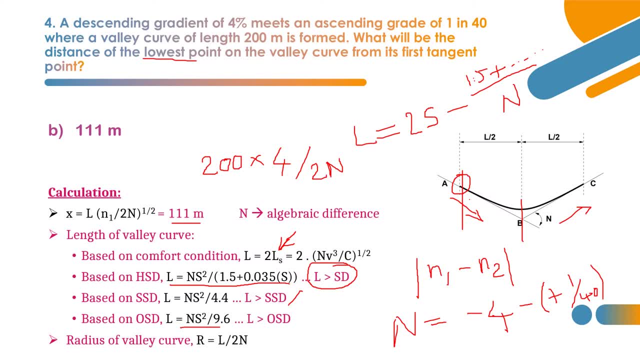 and for osd, l is equal to n square by 9.6. when l is less than osd, it is 2s minus 9.6 by n. how to calculate the radius of valley curve given by this formula: radius of valley curve is: 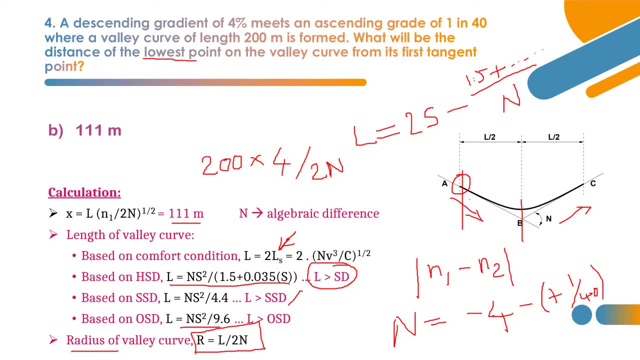 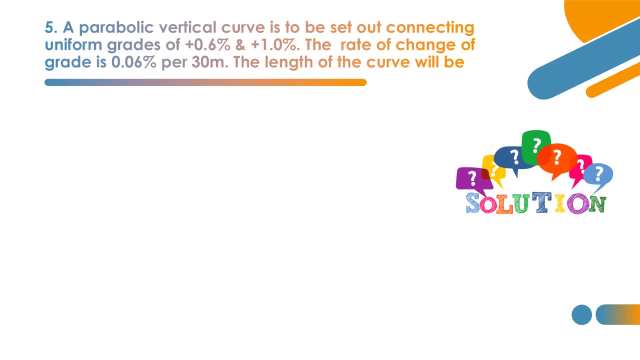 capital l. that is the length of valley curve divided by 2n. so this is a. these are some important points about valley curve calculation. now let's see a fifth question. a parabolic vertical curve is to be set out connecting uniform grades: 0.6 percentage and 1.0 percentage. both are ascending gradients. the rate of change of 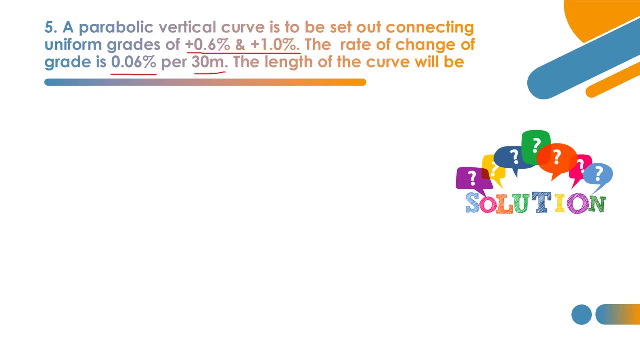 grade is 0.06 percentage per 30 meter, we have to find the length of the curve. this is one easy logical problem: you have to calculate. so they have given the rate of change of gradient as 0.06 percentage per 30 meter and two uniform grades. both are ascending. by using this data, we have to find the length. 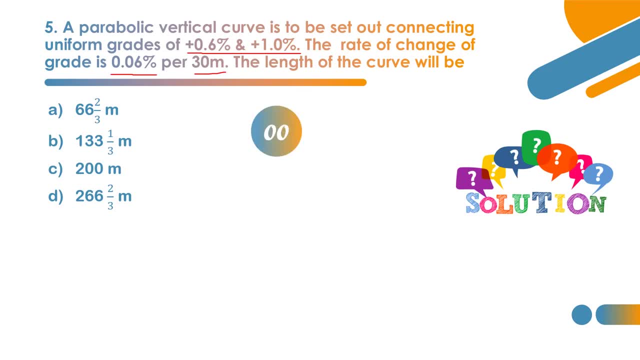 of the curve. this can be solved by using logic, easy one option: c, 200 meter, is the answer. so change of grade is nothing but 1 minus 0.6 capital n. or we can say: deviation n is 1 minus 0.6, so 0.4 percentage and rate of change of grade is 0.06 percentage per 30 meter. for 0.4 percentage, what is the length? so 0.4 divided by 0.06 into 30 gives the answer as 200 meter. so this is a simple problem. now let's see more about grade compensation. so grade compensation is not needed for gradients flatter than 4 percentage. this is as per irc code and when. 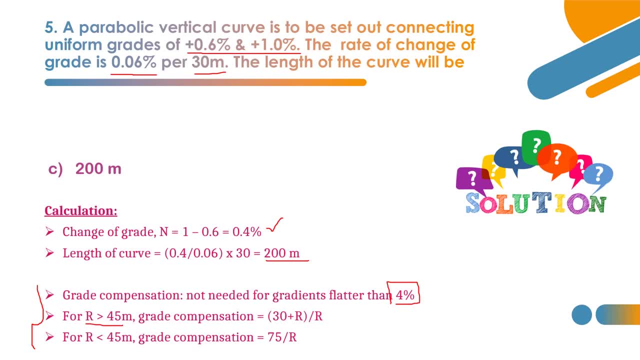 the radius of horizontal curve is greater than 45 meter grade, compensation shall be 30 plus r by r. and what is the compensated gradient? ruling gradient minus the this grade compensation value. and when horizontal radius is less than 45 meter grade compensation shall be 75 plus. 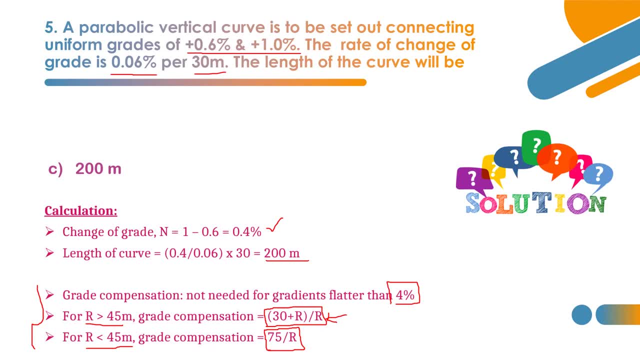 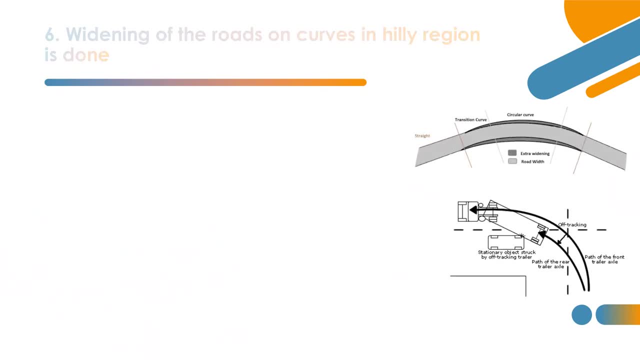 75 by r. so this is how we have to calculate the grade compensation. now let's move on to sixth question. sixth question is based on widening of roads. so widening of the roads and curves. widening of the roads and curves in hilly region. so in hilly region, how it is done. option a on. 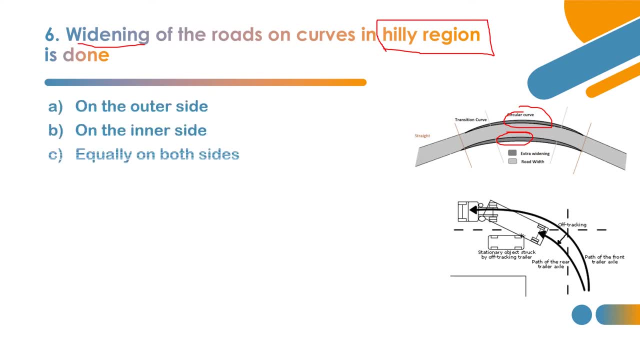 the outer side alone. option b on the inner side. option c: equally on both the sides. option d: less on outer side, more on inner side. so what is the correct side or correct representation for construction of widening of the roads, whether it will be widening on the outer side? 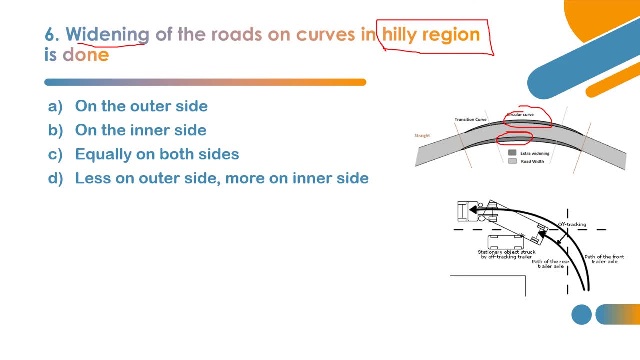 only, or inner side only, or equally on both the sides, or less on outer side and more on inner side. in hilly region that is the main thing. so in hilly region widening of roads is done on the inner side only, not on the outer side or equally on the inner side only. 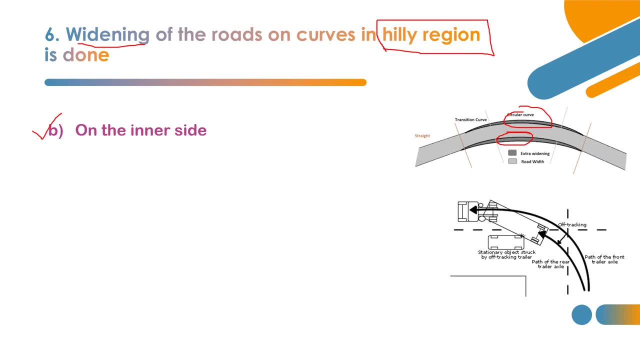 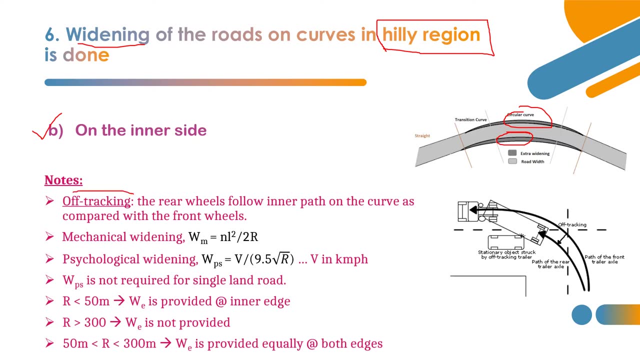 widening is done only in plain regions. both the sides are done. now let's see more about it. why widening is done? because of this off tracking phenomenon. so what is off tracking? the rear wheels follow inner path on the curve. so you can see in this diagram this is rear wheel, so that follow. 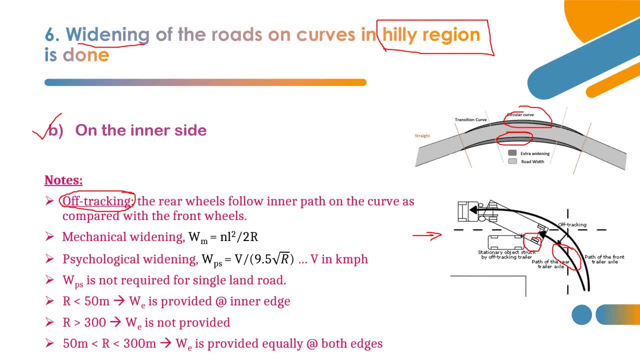 what inner path on the curve. so this is the inner path, so that rear wheel follows the inner path on the curve as compared to front wheels. this is the front wheel and this is the rear wheel. so you can see in this diagram clearly real rear wheel follow the inner path as compared to front wheel, front wheel is correct, correctly. 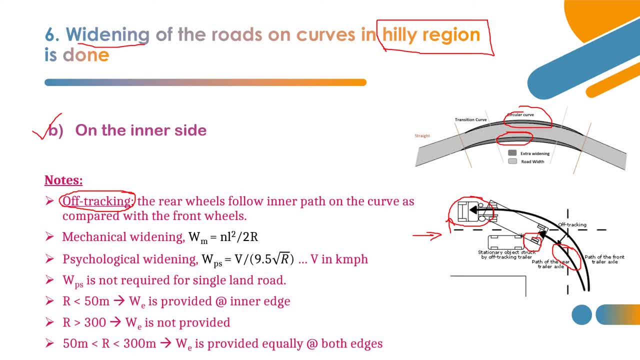 projected, but rear wheel is not. so that's why widening is given mechanical. there are two types of widening: mechanical and psychological. so mechanical widening is given by this formula: this is nothing but the off tracking formula. n. l square by 2, r, n is nothing but number. 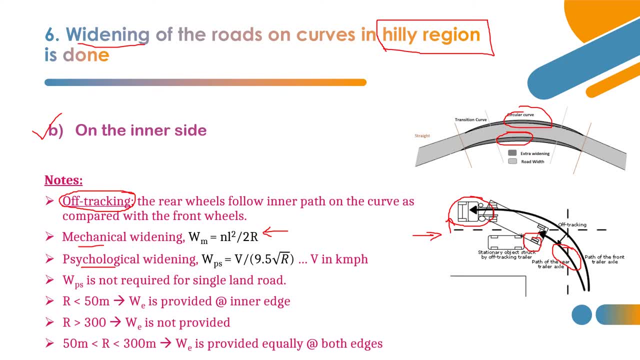 of lanes in the highway. so n l square by 2 r, l is nothing but the length of wheelbase divided by 2 r. r is radius of curve. psychological widening is given by this formula: v by 9.5 root r. here v has to be substituted in kilometer per hour, v by 9.5 root r. wps is not considered for. 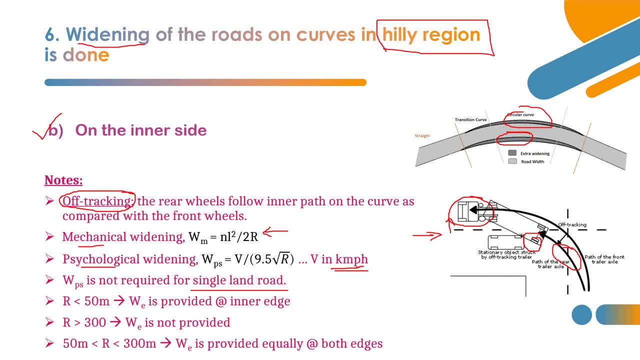 single lane road. so only in multi-lane roads. multi-lane roads are considered, for single lane roads are considered just in case. for single lane road psychological widening is not considered, only wm is enough, and based on the radius of horizontal curve, how widening is provided. when horizontal curve radius is 50 north, then extra widening is provided at. 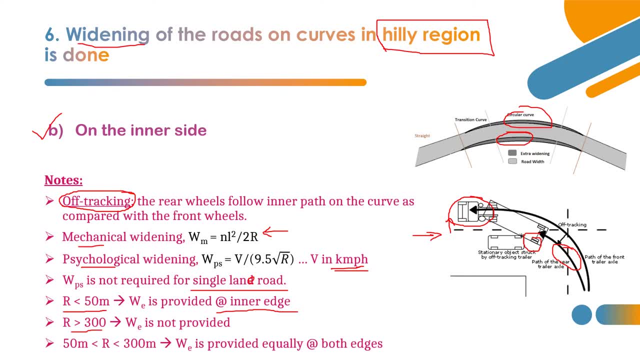 inner edge only when it is greater than three hundred meters. phi is not required when it is between 5, 50 and hadsee parts. width of the land is required, then extra widening ir gear into the one pieceburkh when it is smaller than 300 meters. 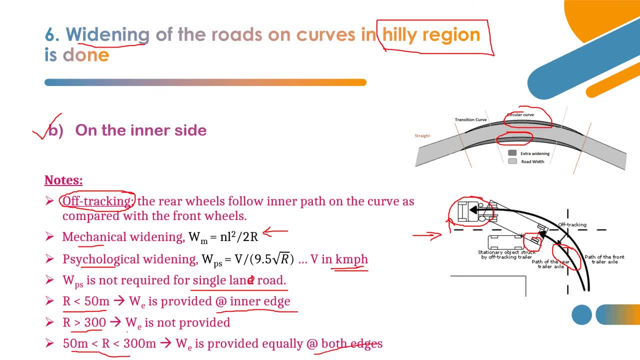 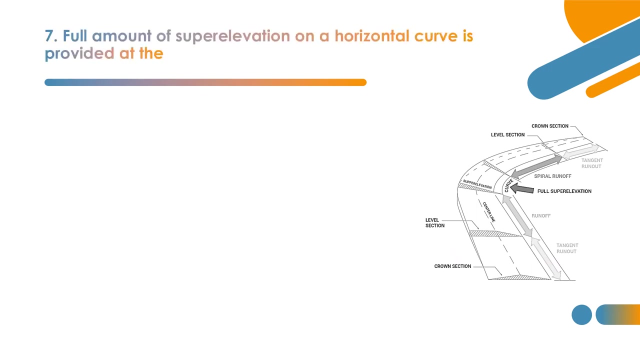 to 300, then extra widening is provided equally at both the edges. so, equally at both edges. extra widening is provided even in case, uh, in case- of hilly region. widening is provided on inner side only. now let's move on to seventh question. full amount of super elevation on an horizontal curve is provided at the though this question 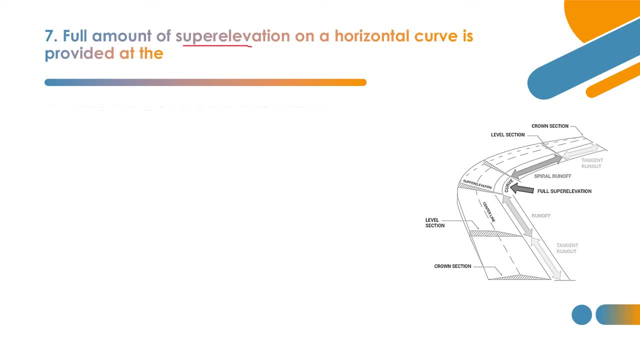 is purely based on super elevation: option a- beginning of the transition curve. option b- center of the circular curve. option c- end of this transition curve. option d- center of the transition curve. so full amount of super elevation is provided at which location you can refer this diagram to give to get the correct answer whether it is so. beginning of transition. 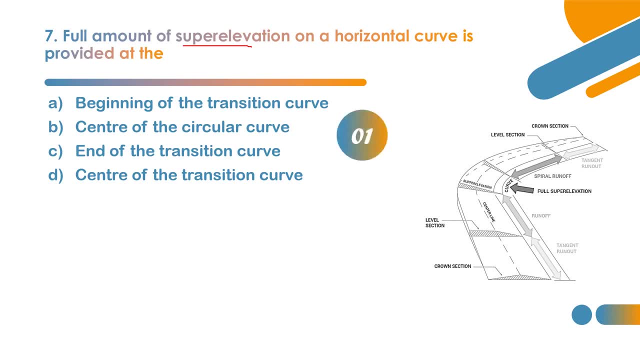 curve, or center of circular curve or end of transition curve or the center of transition. so the correct option is option c, end of transition curve. you can see in this diagram super elevation is gradually provided like this and reach the maximum at here. so this point, super elevation, is reached fully. so what is that point? the beginning of the circular curve. 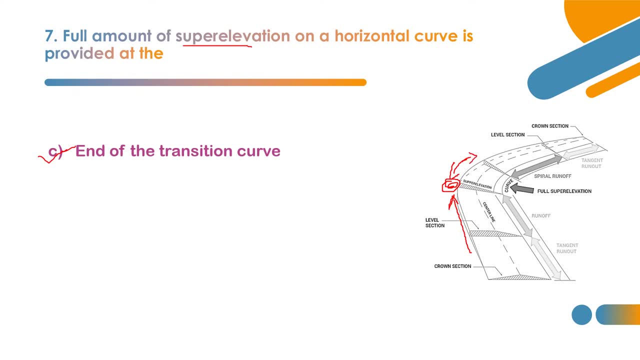 this is the actual circular curve. at the beginning of the circular curve, super elevation is attained at maximum. that means, uh, actually, this is the circular curve and this is the transition curve. these are the transition curve. so circular transition curve, this is transition, this is circular. so at the end of the transition, or we can say, at the beginning of circular curve. 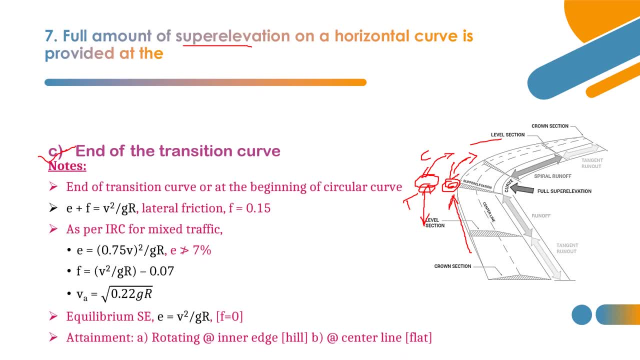 super elevation is provided full amount. let's see more about super elevation and its calculation. e plus f is equal to v square by gr is the basic formula for the super elevation, where f is the nothing but lateral friction coefficient. here f is lateral friction but in ssd calculation that coefficient of lateral friction coefficient. 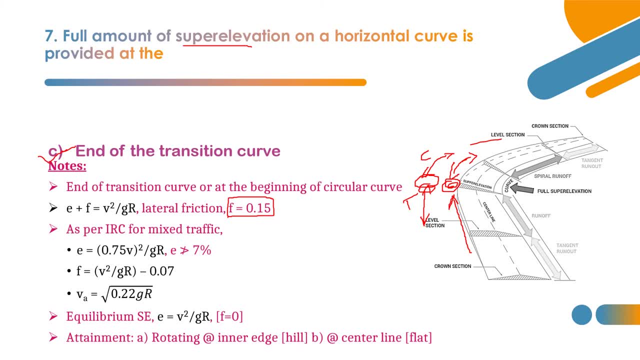 of friction will be based for longitudinal, not lateral. so that's why their f value will be some point: three, six, one, three, five, like that, here lateral friction, here lateral friction. lateral means, uh, like this, perpendicular to the direction, perpendicular to the movement. so lateral friction is: f is equal to 0.15, typically. so e plus f is equal to v square by gr. so as per irc, these three 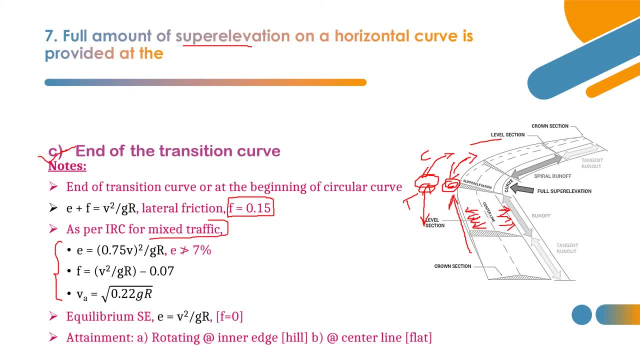 formulas are followed for a mixer traffic condition or mixer traffic condition is equal to 0.75 v. square v, the whole square. this is uh. this square is not uh for only velocity. this is a whole square. 0.75 v, the whole square, divided by gr. whenever small v comes, this is for meter per second, only capital v. 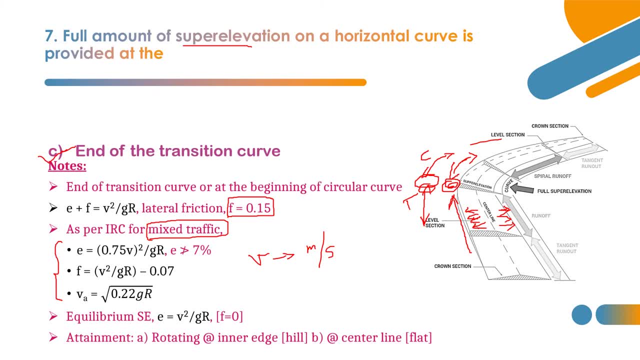 means kilometer per half, and another formula for lateral friction is v square by gr minus 0.07, because e shall not be greater than seven percentage and uh. in case of snow roads it can be maximum up to 10 percentage. in case of normal roads it can be. it shall not be greater than. 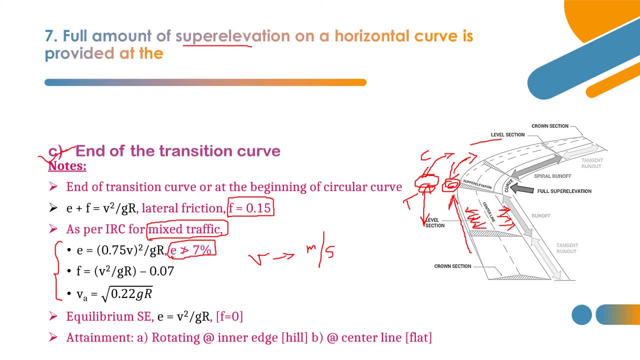 it shall not be greater than seven percent. so that's why f is equal to v square by gr minus 0.07, and this is the allowable velocity formula, allowable speed: v suffix a is equal to root of point two to zero. so these three formulas are based on irc and irc, and, and it is meant for. 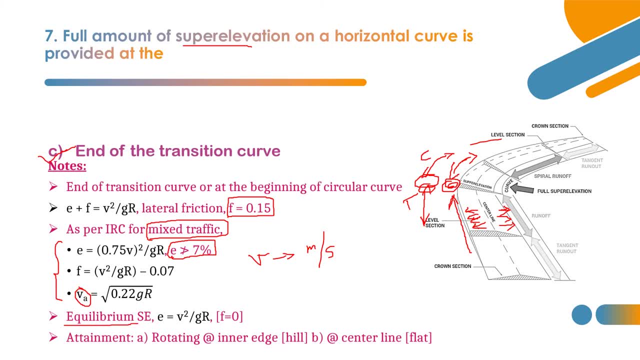 mixer traffic condition and there is one concept called equilibrium super elevation. that means we are, we are not uh, considering the friction value, only uh, we consider there is, there exists no friction. that is f. f is equal to zero. so that means that super elevation is equilibrium in condition. so equilibrium super elevation given by this formula e is equal to v. 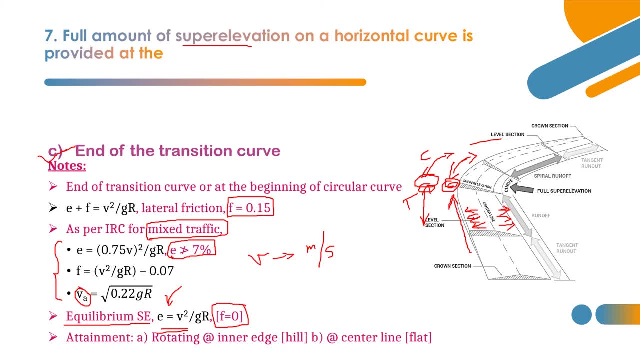 square by gr, without considering the lateral friction. and how super elevation is attained. there are two methods: by rotating about inner edge, by rotating about the center line, so this is the center line. by rotating about the center line, we can obtain the super elevation. here in this diagram they have attained this super elevation about inner edge, so this is the inner edge. so 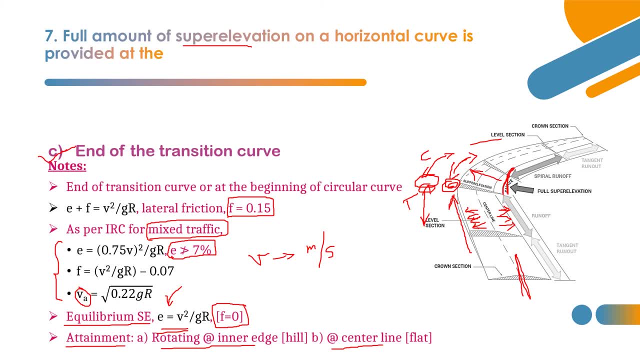 super elevation obtained like this: rotating about inner edge. when, uh, in case of hill, rotating about inner edge is followed, in case of flat terrains, rotating about center line is followed. so there are two applications. now let's move on to eighth question. horizontal curve of radius r is equal to 260 meter on a two-lane road, two-lane two-highway. 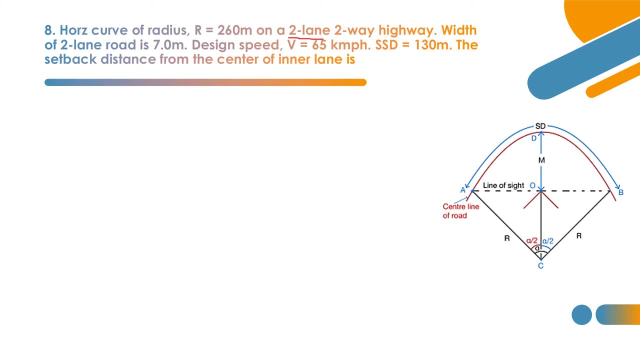 width of two-lane road is given as seven meter, design speed is given a 65 kilometer per hour and stop stopping side distance, ssd is 130 meter. we have to calculate this setback distance from the center of inner line. so every point is important, every word is important. 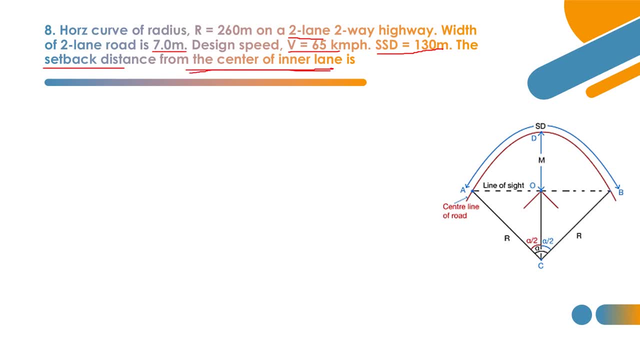 so we have to calculate the setback distance from the center of inner line. so every point is important, every word is important. so options are: a, 8.14, b, 7.14 c, 5.14 meter, d, 9.89 meter. so what is the setback distance? 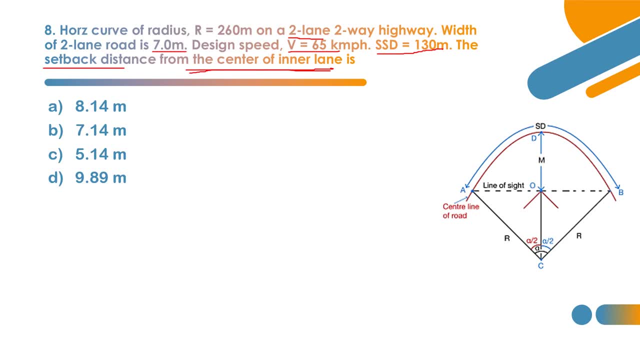 you can refer this diagram to get the. to get what is the setback distance, just pause the video and calculate by using correct formula and check the answer. so the correct option for setback distance based on this criteria is option a, 8.14. now let's see how it is calculated. 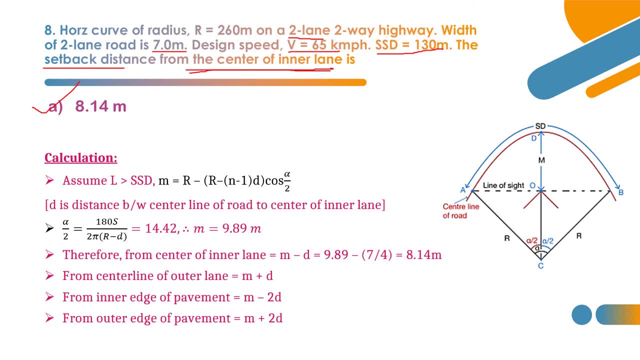 so first we have to assume length of curve is greater than ssd. so by assuming that we get this formula, m is equal to r minus r, minus of r minus n, minus 1, d, cos alpha by 2.. so what is r? we know radius of curve and what is n, number of lanes here, two lane road, so two minus. 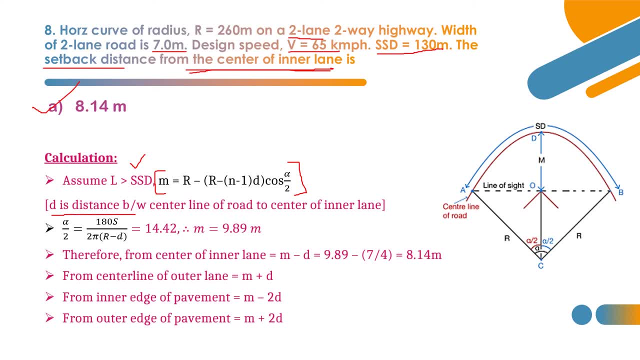 one one. what is d? d is nothing but distance between center line of the road to the center line of center of inner line. so let's see what is that. so consider this as their two lane, two way road. so here, what is the small d value between center line of the road? so this is the center line of the road, this is the center line. 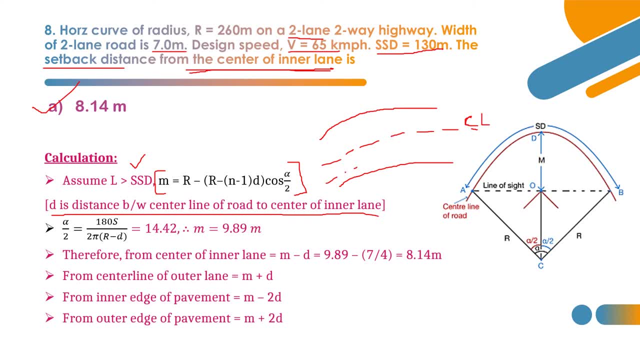 of the road to the center of inner lane. so let's consider this as the center of inner lane. so this distance is nothing but small d. so this distance is small d. now we have to calculate alpha by 2 value. so that will be calculated by using this formula: alpha by 2 is equal to 180 s by 2 pi. 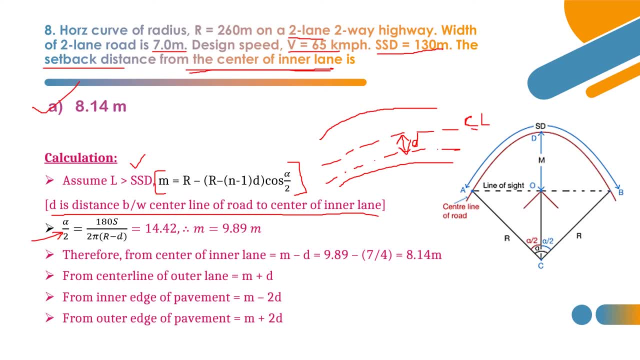 minus d. so what is s side distance? they have given 130 meter. so by using this formula we get the answer, for alpha by 2 was 14.42 and that value will be substituted here so that we can we get the value of setback distance and this setback distance. 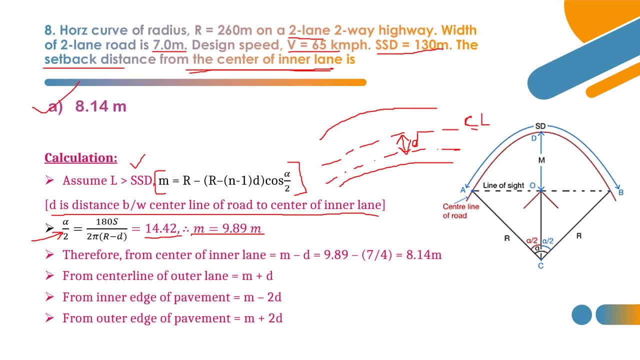 is a distance from center of the highway, center of the road. you can see in this diagram here what is center line of road. so from that m value is got, n value is obtained as 9.89 meter. you may see in the options option d is given as 9.89 meter but in the question they have asked for setback. 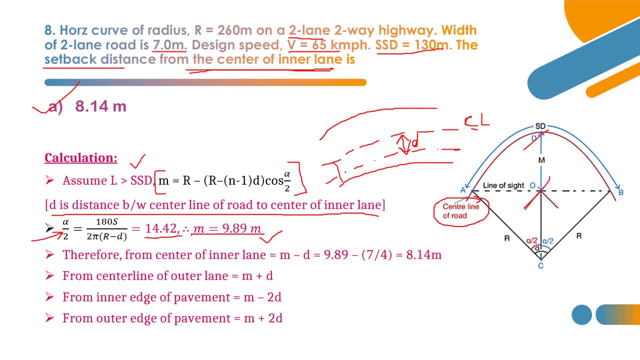 distance from the center of inner lane. so this is the inner lane, so we have to calculate setback distance from this value. we have to calculate setback distance from this one: this is the center of inner lane. from this we have to calculate setback distance. so for that we have to. 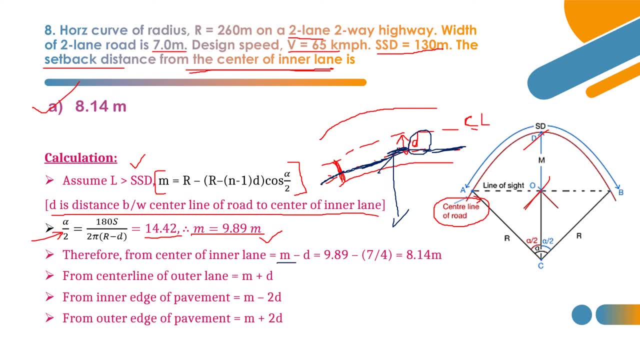 minus the small d value. so that's why m minus d is calculated to get the answer for setback: distance from center of inner lane, center of inner lane to the line of sight. So how to calculate small d value? It is nothing but 7 by 4.. What is 7?? Width of the. 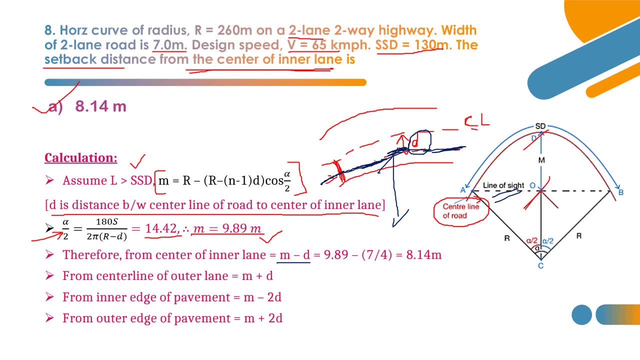 two-lane road, So small. d is 4 times small. d gives the width of the line, width of the road, So small d value is 7 by 4.. We can calculate like this: A minus d value gives answer as 8.14.. 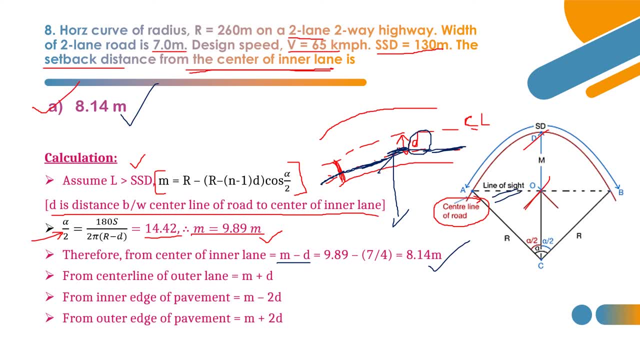 So option is A. So what about other cases? If it is asked for center line of outer line, then m plus d. So this is the center line of center of outer line. So here one small d will be there. So that is why m plus. When it is asked for inner edge, this is the inner edge. 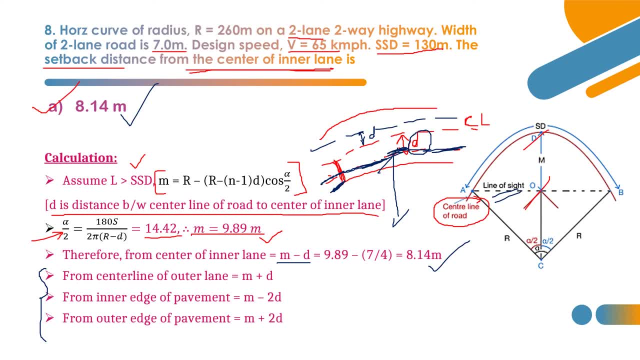 This is the inner edge. Then we have to add one when we have to subtract two d's: Here one d and here one d. So this is the inner edge, So this is the inner edge. So this is the inner edge. 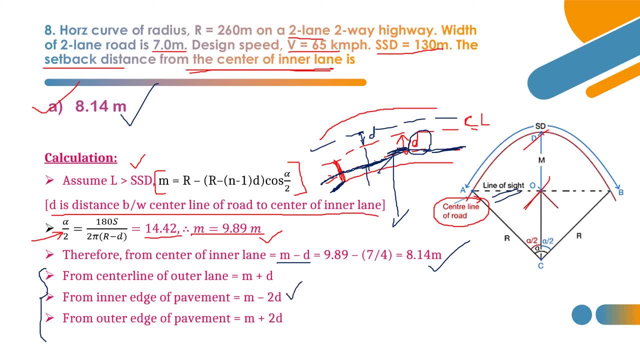 So that is why minus 2 d. When it comes to outer edge, this is the outer edge, So we have to add this d as well as this d. So that is why plus 2 d. So that is why plus 2 d. So this is how we. 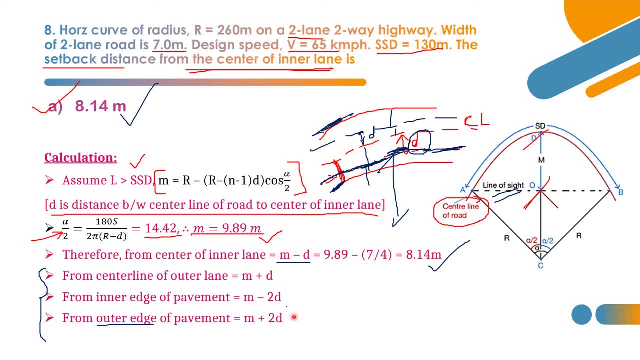 have to specify the answer based on the given criteria. So basically we are finding the value of setback distance from the center of highway. This is the center of highway or center of road, But in the question they have mentioned from center of inner line. So that is why m minus. 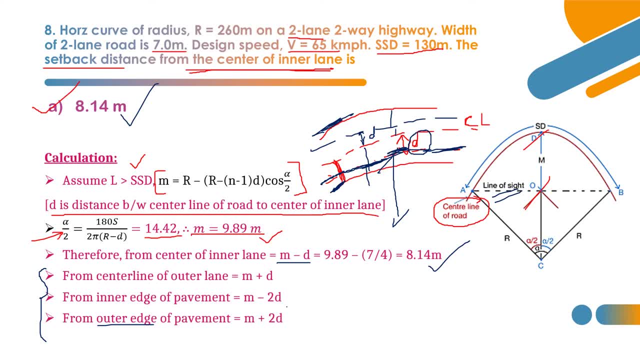 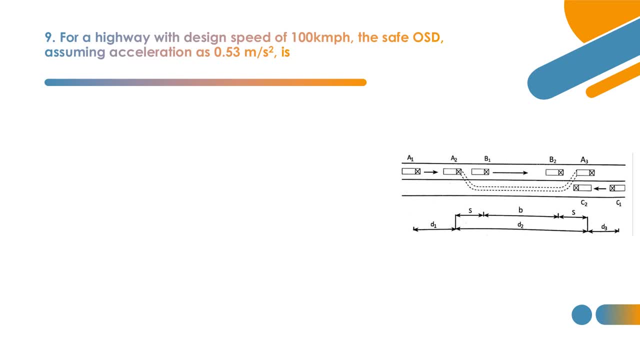 d. Now let us move on to ninth question. This question is based on OST calculation, one important concept in highway engineering: OST overtaking side distance. They have given the design speed of the highway and the acceleration as 0.53 meter per. 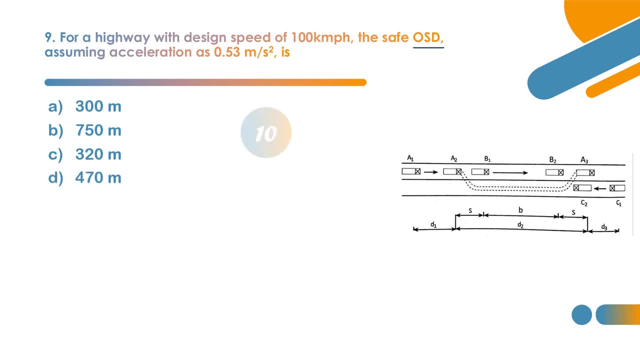 second. So these are four options to get the answer for safe OST value. So there are some two to three calculations involved in this OST concept. You can pause this video and get the answer and check it. So the correct option is option d. 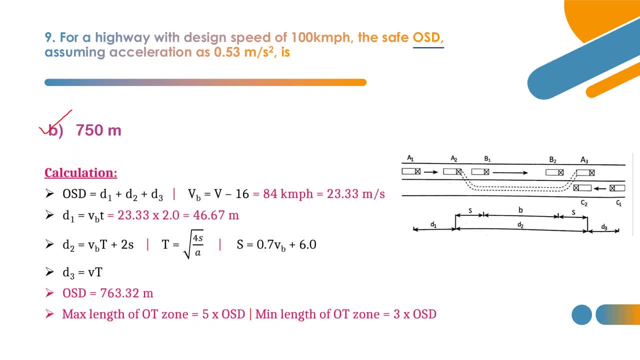 750 meter. Now let us see how it is calculated Basically. OST formula is the summation of these three distances. What are those? d1, d2 and d3.. So d1 is given by VBT. What is VB? VB is: 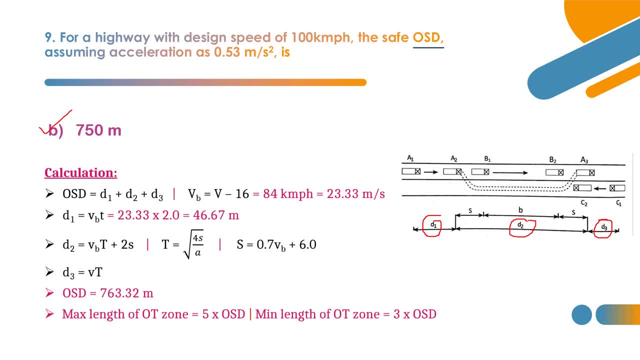 nothing but velocity of overtaken vehicle. velocity of overtaken vehicle, That is velocity of this vehicle. This vehicle is the overtaken vehicle, This vehicle is the overtaken vehicle, So this vehicle has the velocity VB. So velocity of overtaken vehicle into time reaction. 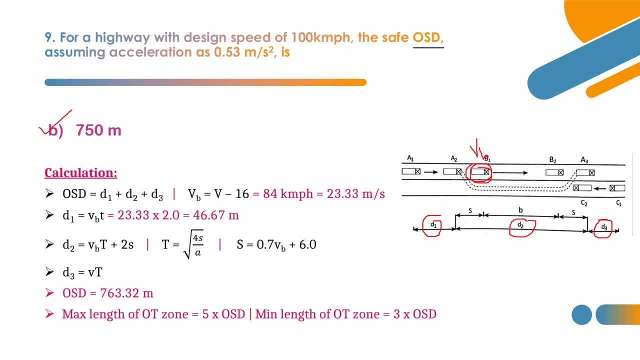 time. Basically in calculation for OSD we take reaction time as 2.0.. But in case of SSD calculation- stopping side distance- we take reaction time as 2.5 seconds. Please note it, because in SSD we take 2.5 seconds as reaction time, In OSD we take reaction. 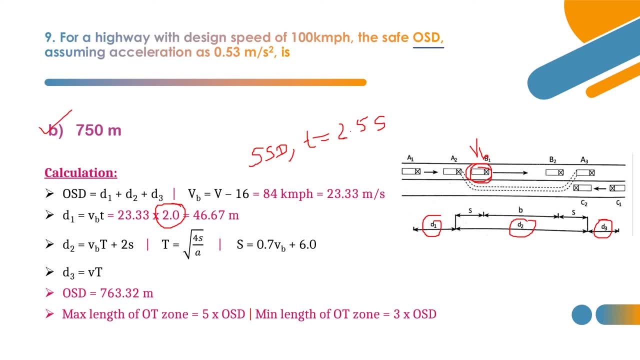 time as 2 seconds only. So that is why VBT is equal to 23.33 into 2.. How 23.33?? We are calculating in meter per second. How it is 84?? Basically overtaking vehicle minus 16. 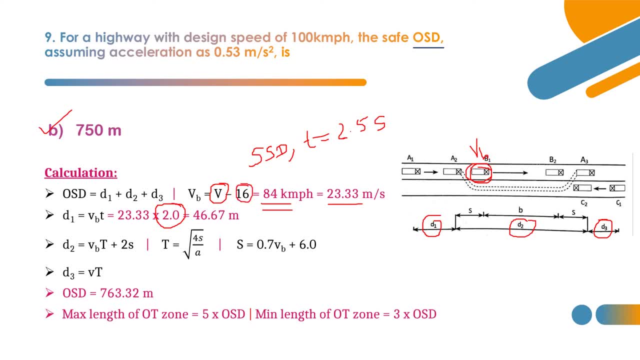 kilometer per hour gives the answer for velocity of overtaken vehicle. This is some general assumption, because when the difference between two vehicles is 16 kilometer per hour, then overtaking can be done. So that is why overtaken vehicle's velocity is nothing but overtaking. 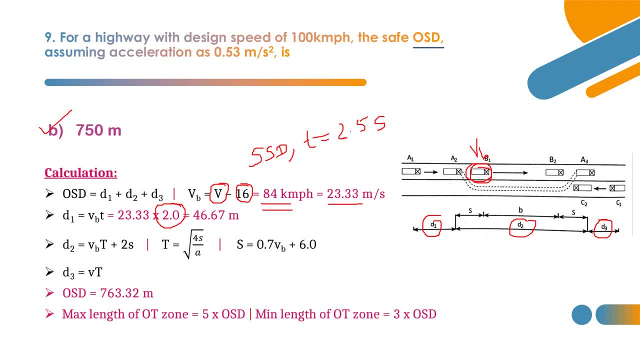 velocity minus 16.. So that gives answer as 84 and that is converted into meter per second as 23.33.. So 23.33 into 2 gives the answer for D1 distance. This is the D1 distance. 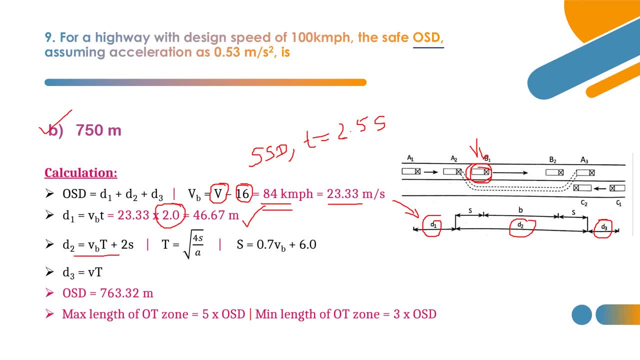 And D2 distance is given by this formula: VB, capital T plus 2S, And how capital T is converted By using this formula: Root of 4S by A, Root of 4S by A, And what is S? Nothing. 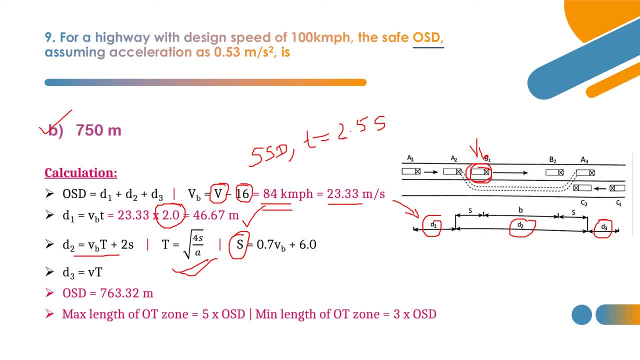 but it is related to the spacing between vehicles And that will be given by this formula: 0.7 velocity of overtaken vehicle. that is, V suffix B plus 6.. 6 is nothing but length of wheelbase. Length of wheelbase is normally 6 meters. In some case it will be 6.1 meters. 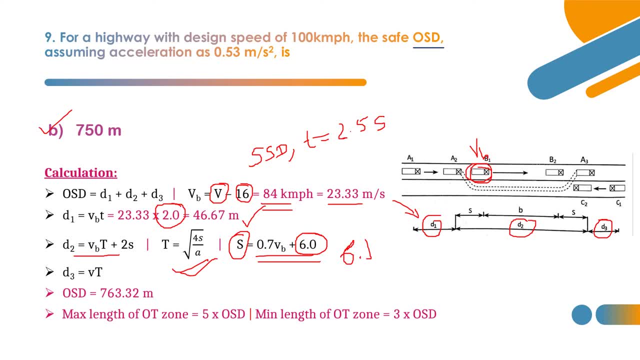 If it is mentioned in question, we have to adopt that only, But in. but normally 6.0 is the length of wheelbase, So spacing is given by 0.7 VB plus 6. And it is small VB. 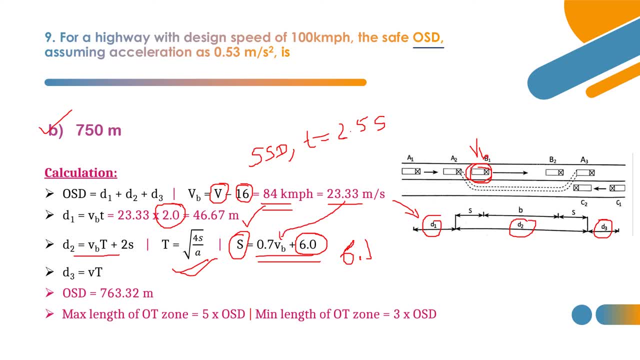 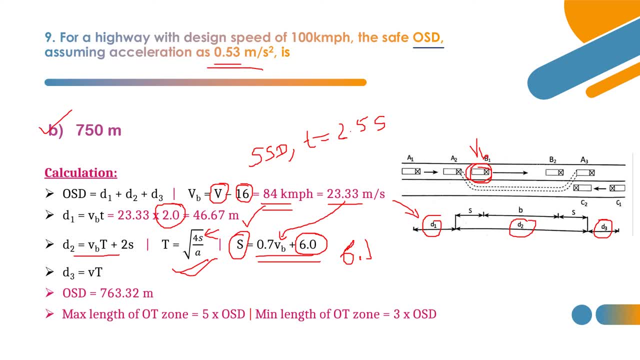 Aeda is given us 0.53 meter per second square. Sometimes acceleration will be given in terms of kilometer per hour per second, So that has to be converted into meter per second square and then that value is substituted over here, So 4 as by a and root of that. 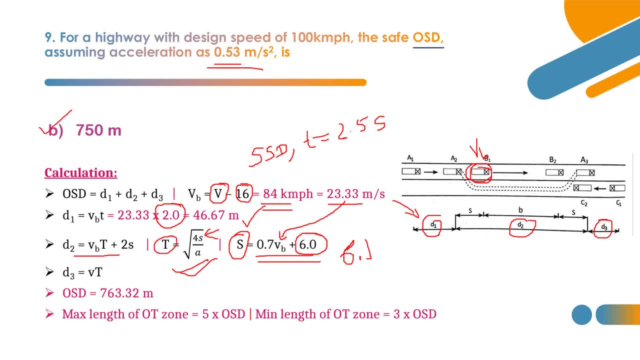 thing. we will give the answer in seconds for capital T time. So VBT plus this capital T is nothing but overtaking time. so VBT plus 2 years gives the answer for what d2? why two times? yes, because here one spacing, here one spacing. so 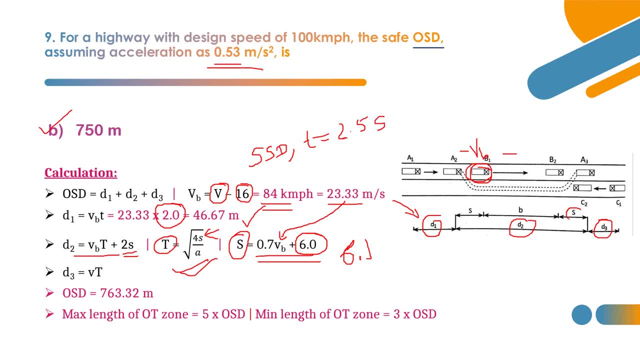 that's why two times yes value. you can see here 2s plus vbt. vbt is this small b. so this is the d2 value and d3 value is nothing but v into t. v into t. here v is for velocity of overtaking. 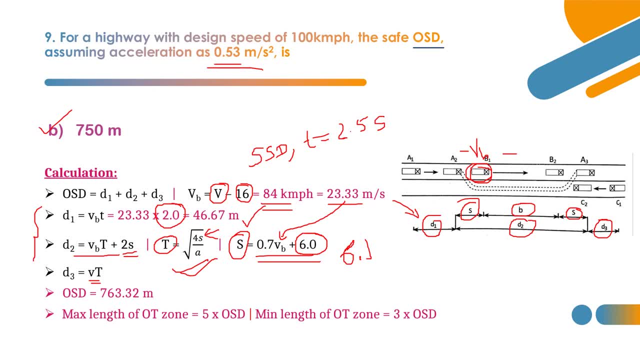 vehicle in meter per second. so this is how we have to calculate every distance value when it comes to a single lane or single way road. one way road, then d3 will not be there, only d1 plus d2. when it comes to two way road, we adopt all the distance value, all the three. 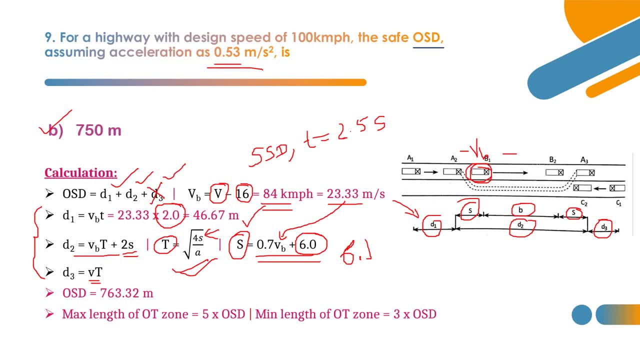 distances. so when it comes to only one lane road, d3 will not be there. but in this question they have not mentioned about the lanes or ways of road, so we are adopting all the distance values by calculating, by summing up d1, d2, d3, we get the osd value as 763.32 and that is approximated to 750 meter as per the given. 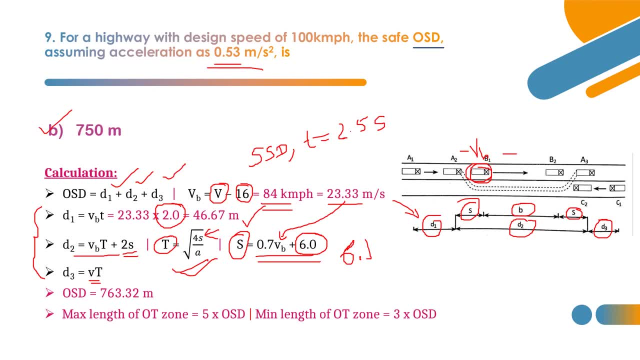 options. so that's why option b is correct. now let's see the other important point in overtaking zone. so maximum length of overtaking zone shall be 5 times osd value and the minimum length of the overtaking zone shall be 3 times osd. so these are the concepts behind osd overtaking. 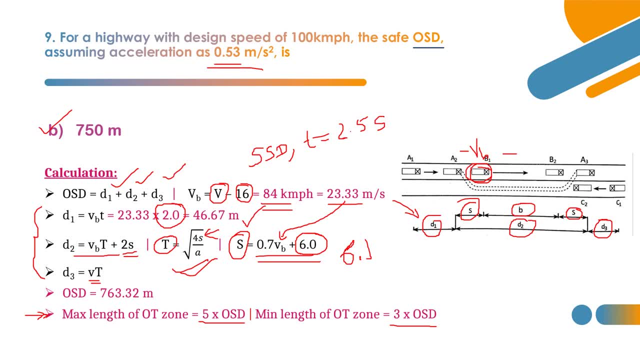 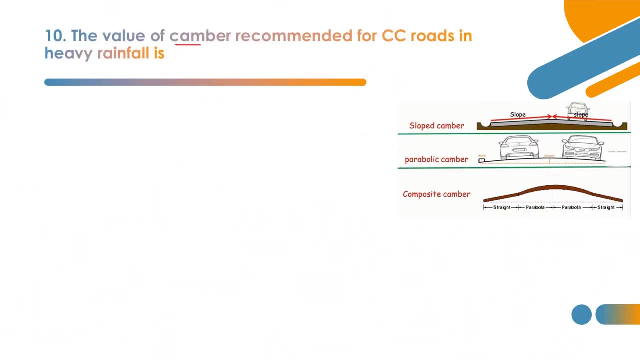 sight distance. this is how we have to calculate osd values. now let's move on to last question, 10th one. this is based on camber. so value of camber recommended for cement concrete roads in heavy rainfall. in heavy rainfall, what is the camber in case of cement concrete? roads, whether it is 1 in 50 or 1 in 40 or less, then this can be calculated as any railing which is in heavy rainfall. if it is in heavy rainfall, then what is the camber? in case of cement, concrete roads, whether it is one in 50 or one in 40 or once in 100 feet, then it 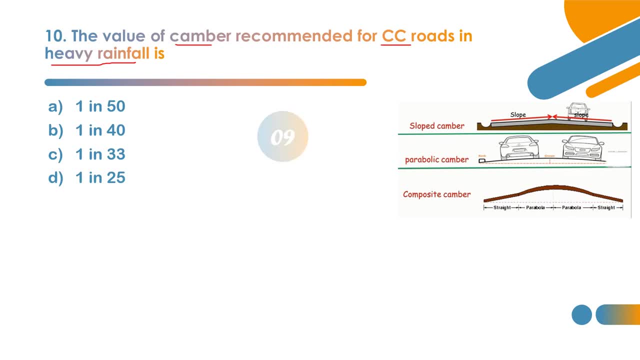 is going to be 1 in 50 or 1 in 40 or once in 300 feet, then this is the camber. it will be 1 in 33 or 1 in 25. so what is the basic value of camber recommended as per irc? 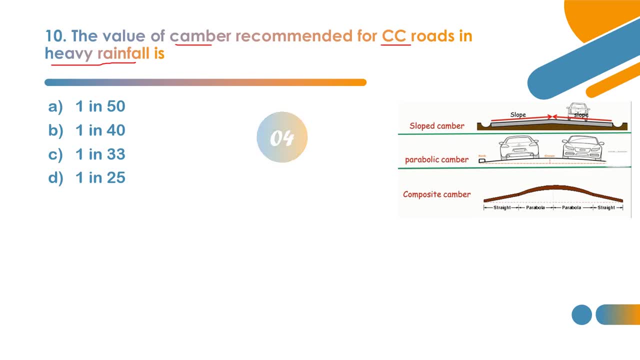 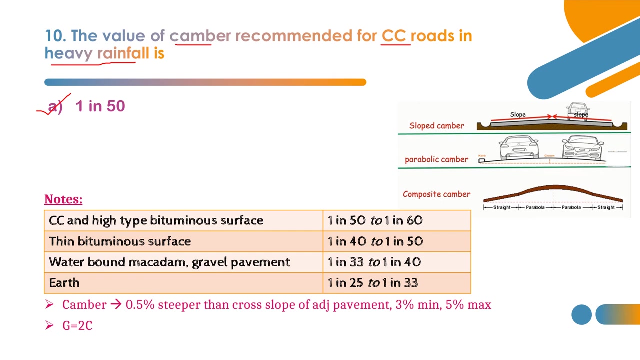 for cement concrete roads during heavy rainfall. in heavy rainfall case, what is the value? so the option is option a, 1 in 50. now let's see some other values with respect to other criteria. so in case of a cement concrete and a high type bituminous surface,